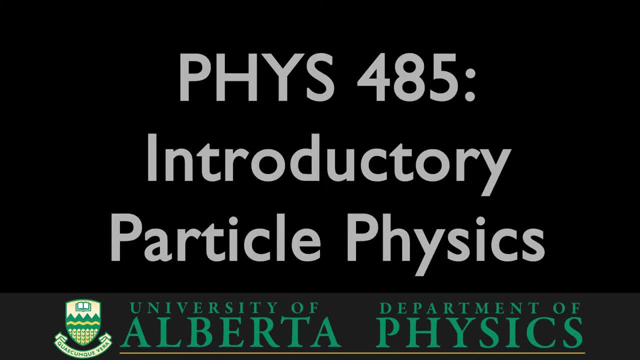 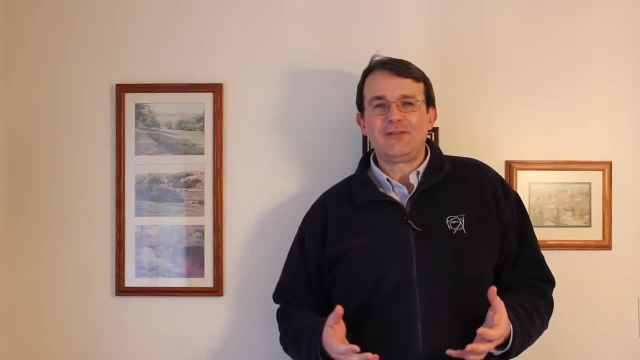 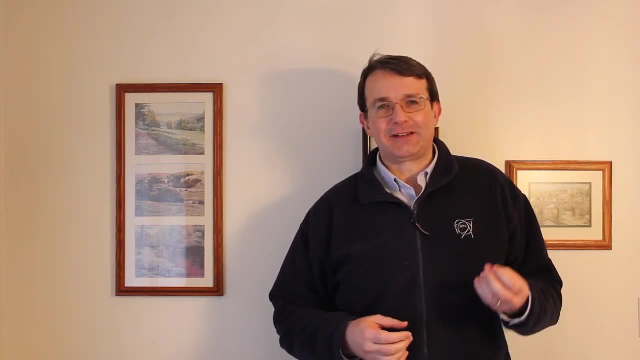 In the previous video we saw how we could draw these Feynman diagrams for quantum electrodynamics, QED. In this video we're going to look at the Feynman diagrams for quantum chromodynamics, or QCD, And where has the QED or? 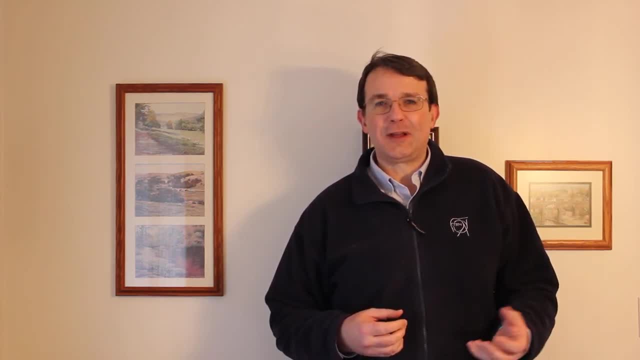 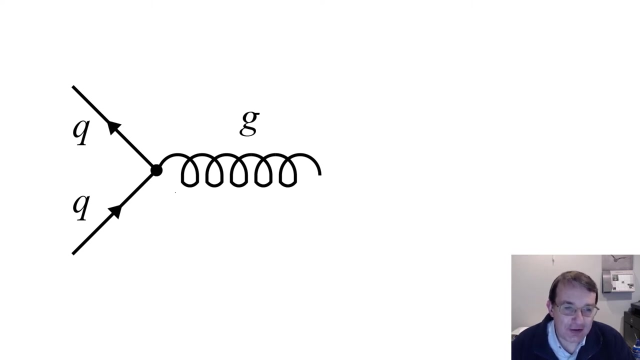 electromagnetism involved all the charged fermions and photons. what we'll see is that for quantum chromodynamics we only deal with quarks and we have gluons. So to see what those diagrams look like, let's switch to the computer. So here we have the basic diagram for QCD and you can see that we have a new. 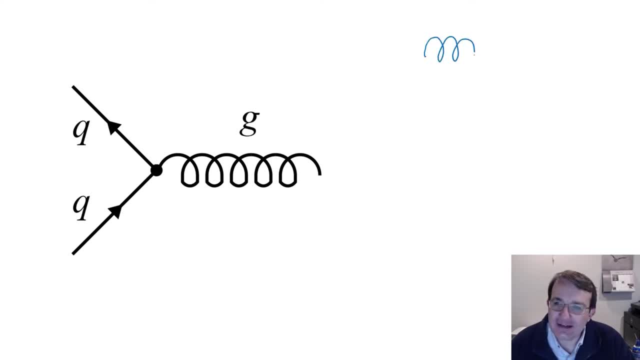 type of line in here and this is the gluon line and it's drawn as if it were a spring, and we'll see exactly why in a minute. So we have a vertex here and this couples using the strength of alpha and s, which is the strong forces coupling. So remember we had alpha, em or just alpha. 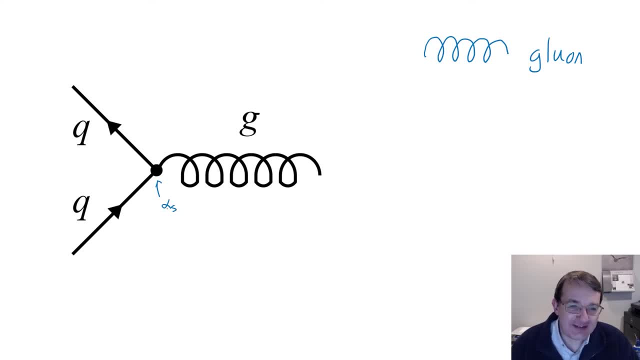 for the fine structure constant for electromagnetism. Well, this is alpha s, it's the essentially equivalent. but now for the strong force. Now, the other difference here is that we're, of course we're coupling to fermion line and we've got a current here, but for the strong force we are limited to only quarks, and 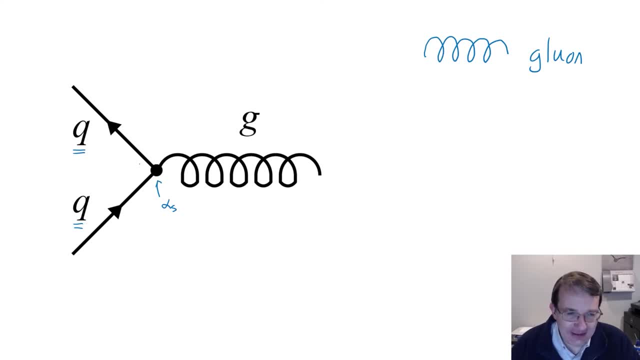 so we cannot have a, an electron or muon or tau in here or any of the neutrinos, because the strong force does not couple to leptons, it only couples to quark. so you can only have a quark line in here, And so this is essentially the same. 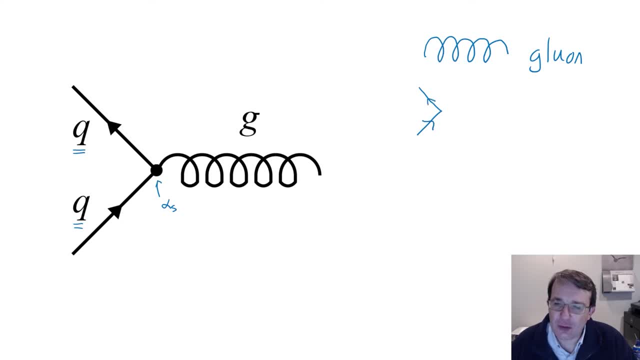 vertex as the one we had for electromagnetism. we had a fermion line coming through here, Fermion, current on that point and firmly coupled to the strong force. So in this example we can only have a new and we had a, a photon right. so this is the qcd equivalent. now, what's going on here is that 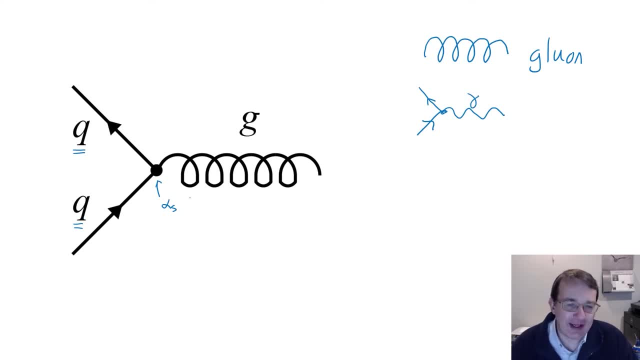 instead of an electric charge we have something called a color charge and you can draw the color charges in. now, we don't draw them in like electromagnetic charges, because, remember, there's three of them. so what you do is you draw what's called a color flow diagram. so, for example, if i 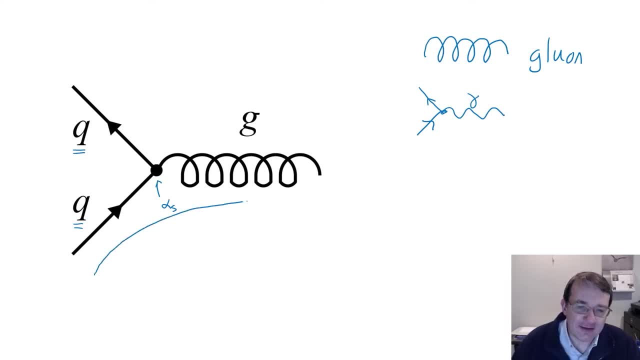 put my pen here, i can draw a line that shows the flow of the blue color charge. so this, for example, is is blue, and for the other side here i can draw in, as you can see now, a red line and i now have a um, so this will be a red here, and so what you can see here is that quarks. 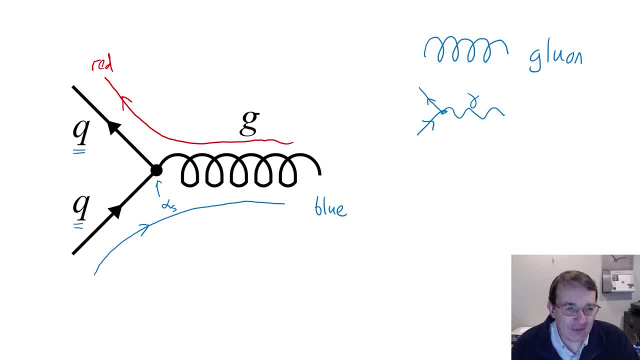 have a single color charge. so here i have a quark that has red color, here i have a quark that has a blue color, and here i have a gluon that is anti-red and blue. and so gluons have two color charges, one anti and one not. you know, uh, i don't know what. 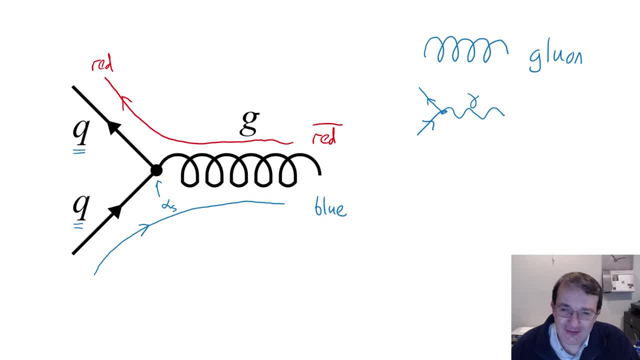 the opposite of anti is non-anti. um. so here we have anti-red blue. you could have blue anti-green or red anti-blue. there's a whole uh, in fact there's eight different uh gluons um that that have these, these mixture of charges. the other point to note here is that we have the same 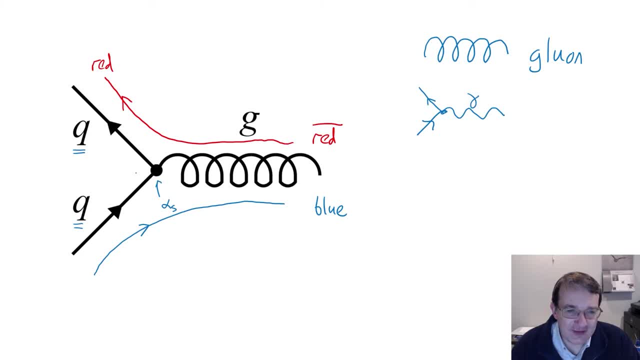 flavor of quark on both sides of this vertex here. right, so we always have the same flavor of quark. so if this was a strange quark, then this would be a strange quark. we cannot have a strange quark here, uh, on the bottom, um. so you know a vertex, something like this is not allowed where you have. 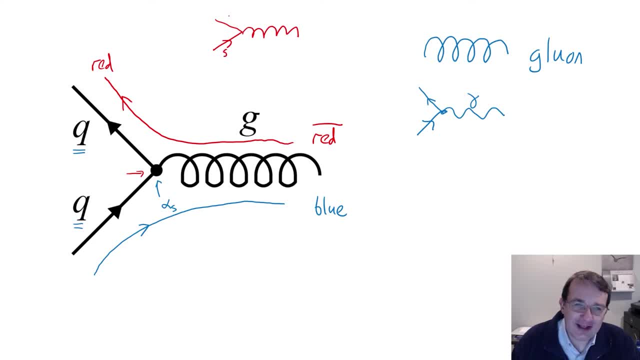 you know, for example, a strange quark and a uh, a down quark. now that would conserve charge, but you cannot have a gluon changing the flavor of the quarks. that is not permitted. so we have these different colors. we have to have the same flavor of quark on both sides of the vertex. 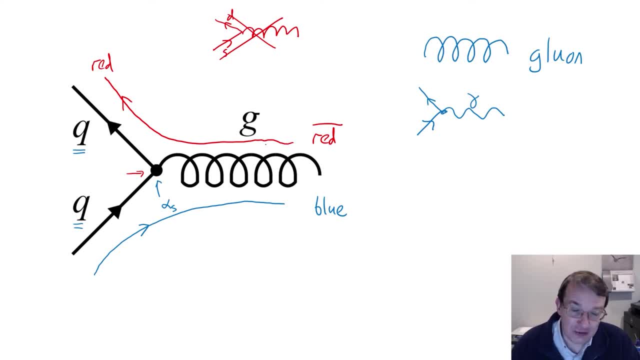 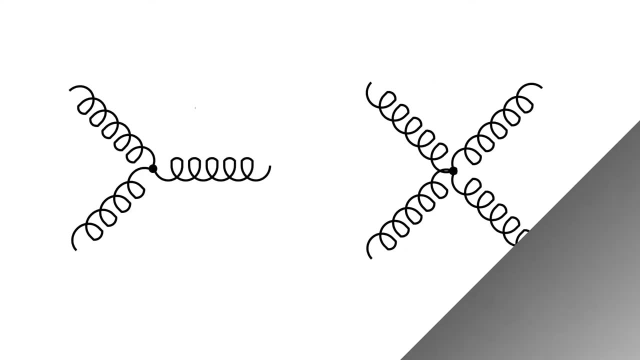 and we have these color flow lines which you can draw in if you like, but, generally speaking, in most cases, unless we need them, we'll leave them off. now, the interesting thing with qcd- and this is the thing that makes it so important to us- is that we have these different colors and we have 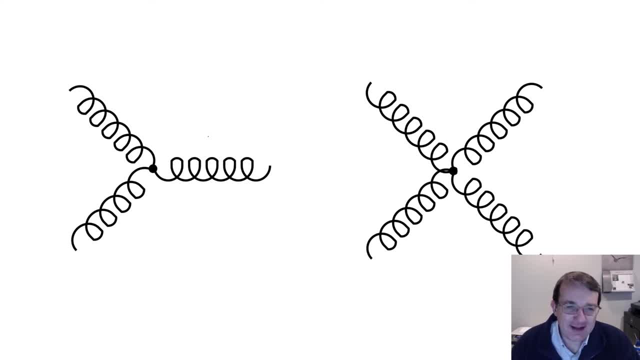 these different colors and we have these different colors and we have these different colors. that different from the electromagnetic force is that, because the gluons have a color charge, gluons can couple to other gluons and so we can have a diagram like this where we have three gluons. so these are all gluons here. 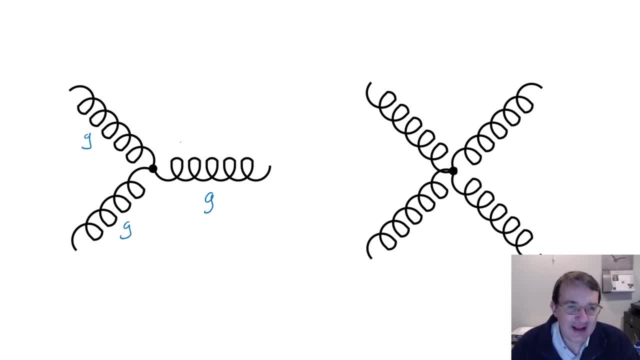 and all three gluons are coupled together and you can draw in color flow. i'm not going to change the color of my pen now, but you can draw in color flow diagrams here such that you know you can see that each of the gluons will have a color-anticolor. 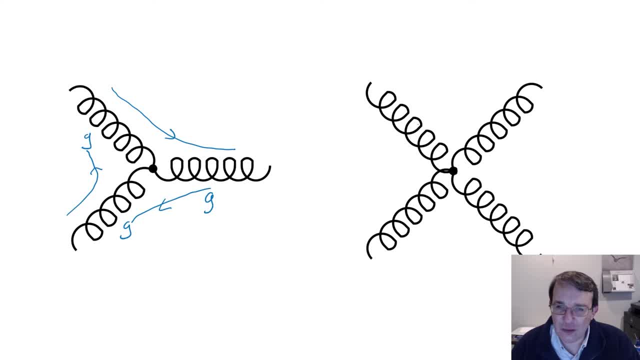 combination, And the same goes on here with our four-gluon vertex, where we have four gluons interacting all at a single point, just like we have three gluons here Now. these diagrams are not possible in electromagnetism, and the reason for that is that the photon carries no electric. 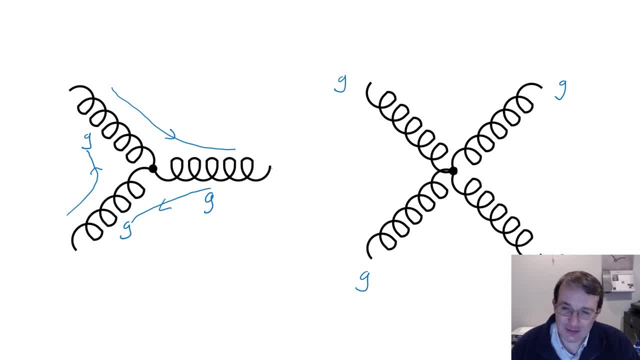 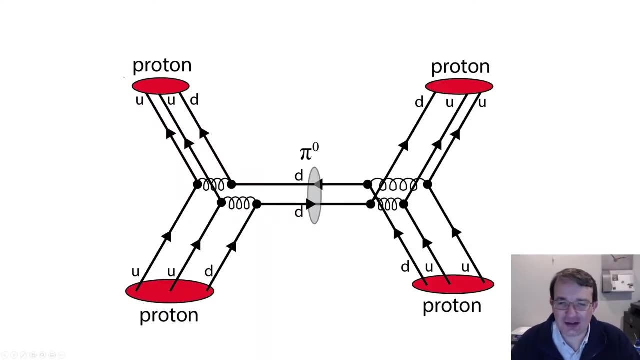 charge, And so the photon cannot interact with other photons, but the gluon does carry a color charge, and so it can and does interact with other gluons. Now, if you remember, we actually discussed, we started our discussion of the strong force quite a few videos ago, when we talked about 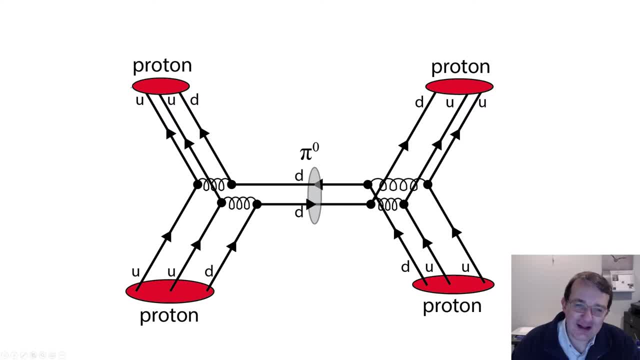 Yukawa introducing these things called mesons in order to explain how two protons were bound together. And so in Yukawa's model there was this idea that we had a proton here and we had a proton here, and they interacted through some exchange of a meson. So now we can actually draw fundamentally what's going on here. 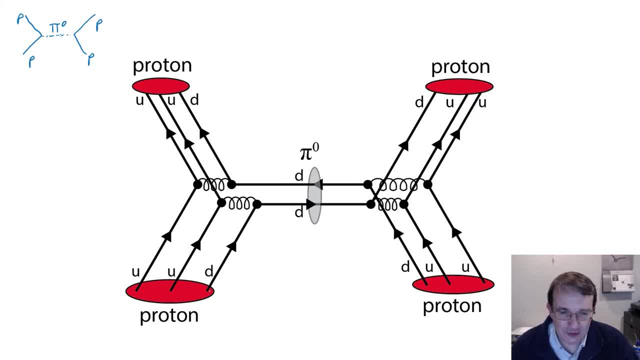 right. Protons are made up of two up and one down quark, all bound together, and so we can draw the protons in here as our three quarks And We can draw these lines going through here. We can have gluon interactions and these produce a down anti-down. 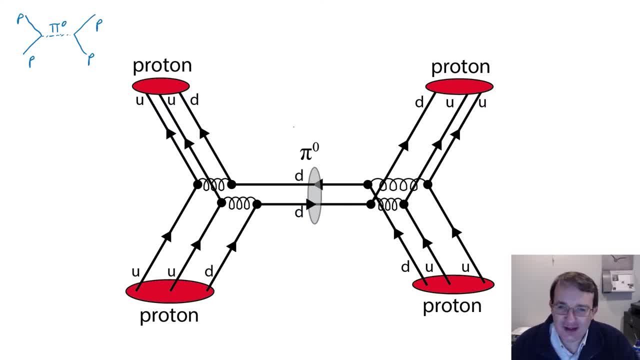 or sorry, this is down anti-down pion that exchanges between another proton over here, And so Yukawa's interaction, that he had as a simple exchange of some, as he thought of it, fundamental scalar meson actually becomes a mechanism that is far, far more complicated than in reality, where we have quarks and gluons. 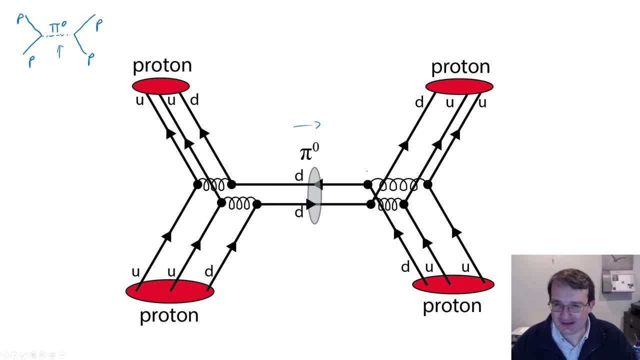 interchanging, forming bound states of mesons and baryons, And so this is actually a sort of a quick diagram of how you can actually implement the Yukawa meson exchange model In the more fundamental understanding that we have now of QCD. 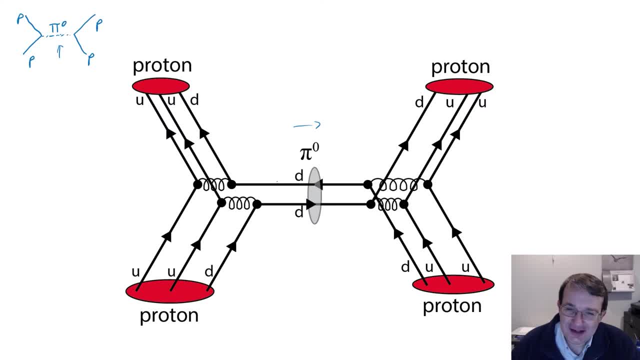 Now, the reason this is also potentially interesting is because in the standard model we have what we regard as a fundamental scalar called the Higgs boson, And in fact there are some theoretical models that solve a problem called the fine tuning problem by suggesting that the Higgs itself may not be a fundamental scalar boson. 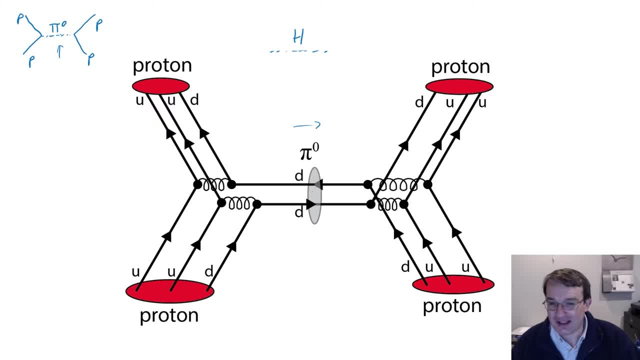 and it may be a bound state, But in fact there are some even more fundamental particles that give us something that looks like a fundamental scalar boson, And those ideas came from, in fact, exactly looking at this Yukawa model, where we originally 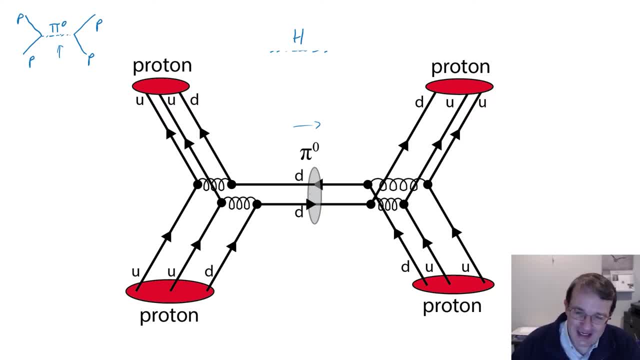 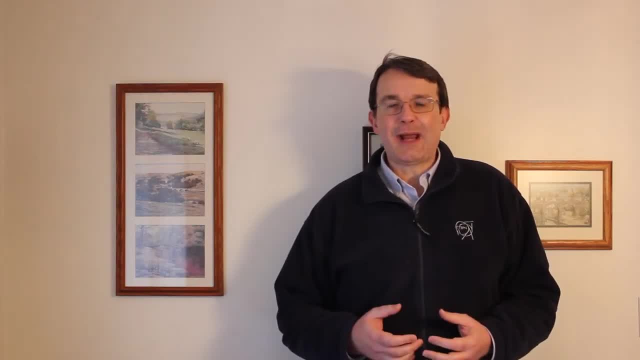 thought there was a fundamental scalar pion And of course now we realize it's not. It's all quarks and gluons. So, like electromagnetism, QCD is a force that comes from a massless vector boson, the gluon. 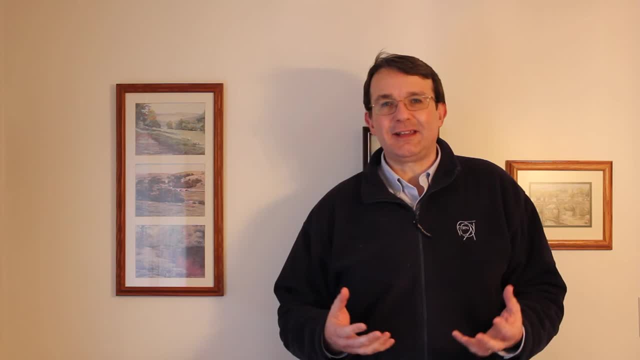 So like electromagnetism, QCD is a force that comes from a massless vector boson, the gluon. So, like electromagnetism, QCD is a force that comes from a massless vector boson, the gluon. So on the face of it, you might think that it's actually going to be very similar to 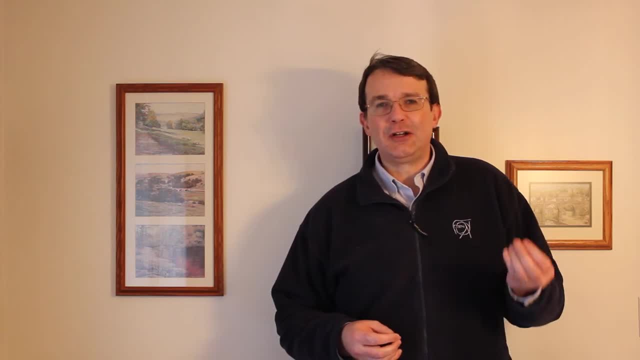 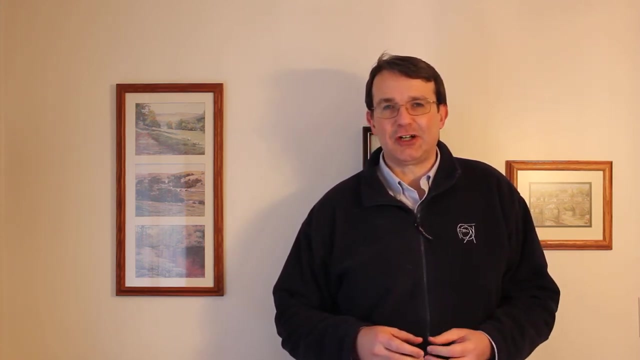 electromagnetism, But, as we saw, the gluon carries a color charge, And so we have these gluon-gluon interaction vertices that simply don't exist in QED, because the photon is electrically neutral, It doesn't carry an electric charge. 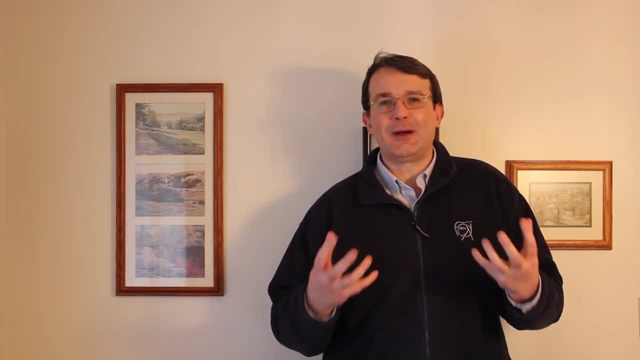 Now, those extra vertices, this extra property where the gluon carries a color charge, are actually a positive charge, Turns out to make a huge difference in the way the force behaves. So let's start by having a look at something that's called confinement. 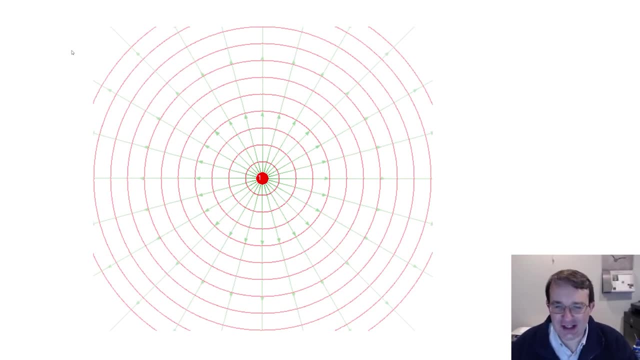 Now to understand confinement, it's good to sort of start by looking at electromagnetism, because electromagnetism is something you're all familiar with and you know how it works. So if what we've got here is we've got a positive electric charge, 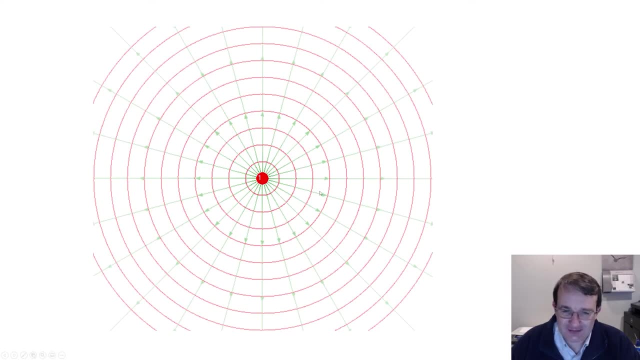 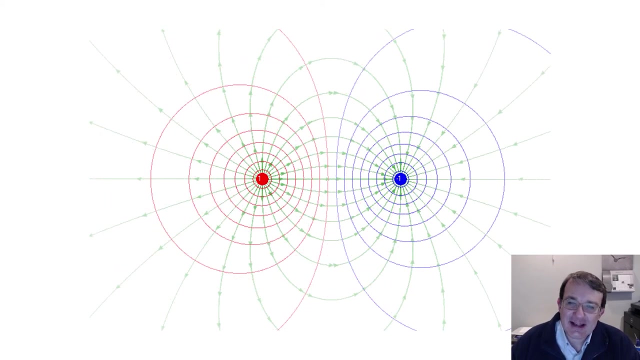 And we've got the positive charge field created by that positive electric charge. Now, if I add into this, I place a negative charge somewhere over to the right, then the field that is then created, as we can see, is the sum of the two independent charges' electric field. 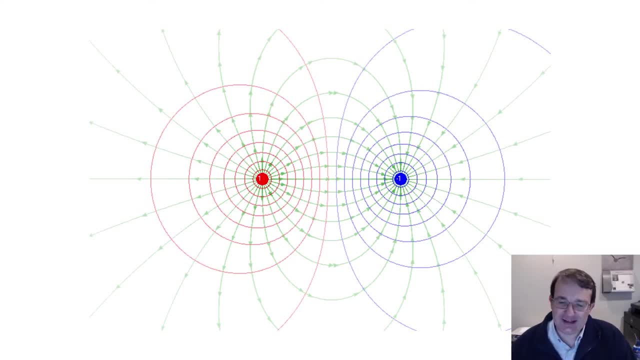 So you can take the electric field of the positive charge, you can take the electric field of the negative charge, and the net electric field is the vector sum of the two independent electric fields. And so, as you can see, we end up with a concentration of field in the middle, here between these two electric 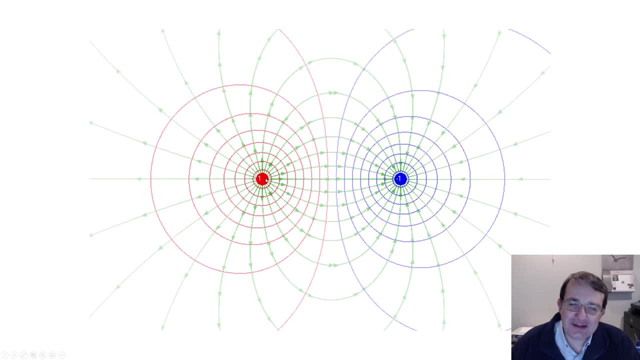 charges. Now if I replace the two electric charges with two quarks and we look at the strong field, then you might expect that you're going to get a strong concentration of field in between the two charges. But of course, just as we see, 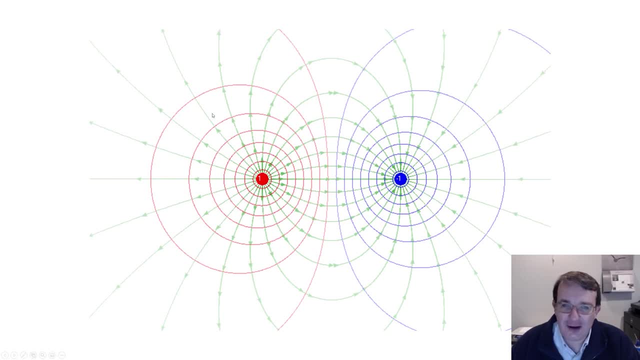 in electromagnetism, you also get this spread of field outside that, However. so this is what you might imagine would happen, is you'd end up with sort of these gluon lines. But the key difference between the electromagnetic and strong fields is that the strong fields are attracted to other strong 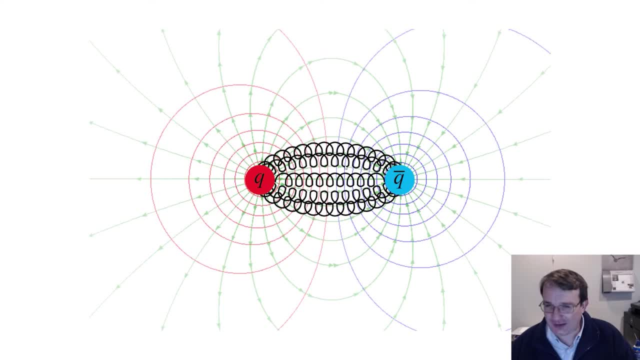 fields. Electromagnetic fields are not attracted by other electromagnetic fields because the electromagnetic field itself does not carry any electric charge. It's only the actual charge that the field interacts with. However, in the case of a color charge, the color field has its own. 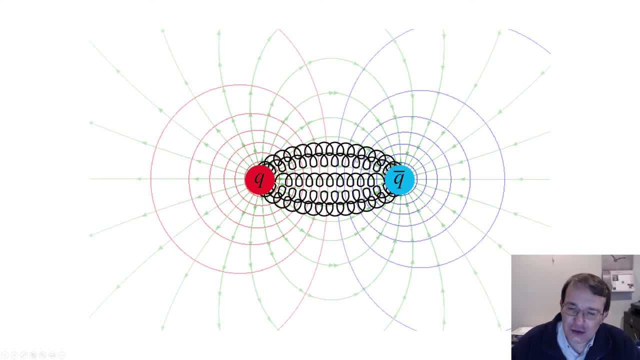 color charge as well, And so the two fields attract each other. And so, while you do start to get this sort of strong region of field in the center, this field attracts itself and causes it to collapse down into a single string of field between the two, So that when you have two quarks- so here's our first quark- 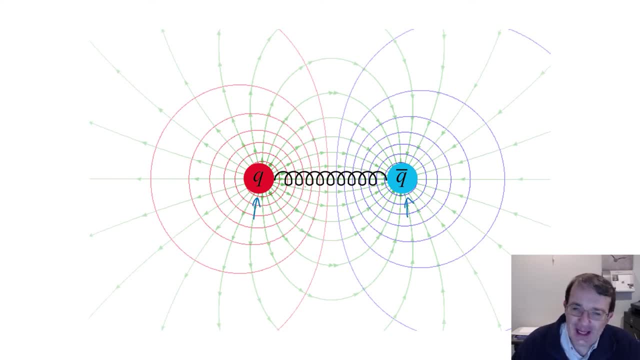 and here's our anti-quark. so opposite charge, what you end up with is a single region of field in between the two. So this is where the entire color field exists, because you know, any field out here is attracted by the existing field and just yanked round and 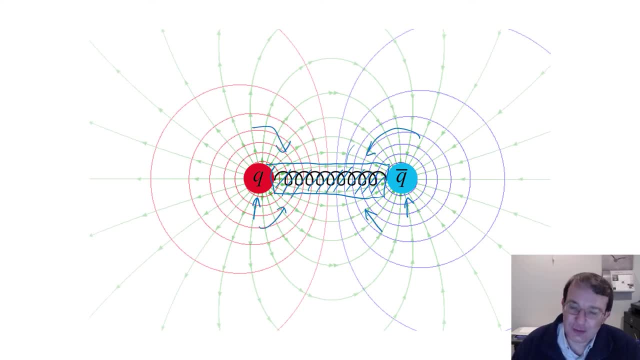 pulled into this one sort of flux tube that contains the entire color field, And in fact that's why the gluon is drawn like a spring, because this tube of force acts, you know, essentially, obeys Hooke's law, You know, as you double the length of it, 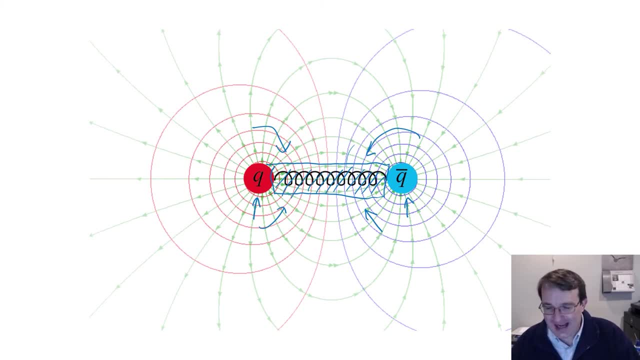 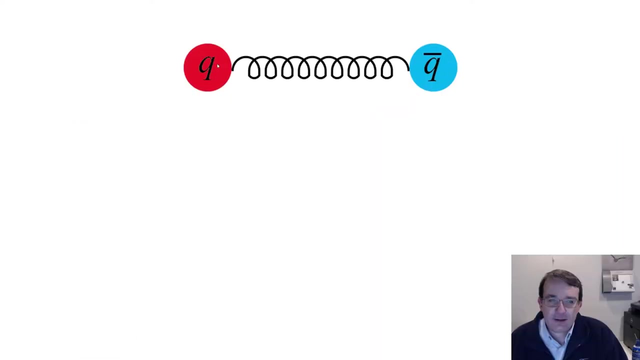 you know, as you double the length of it, you increase the energy in it, according to Hooke's law. you know, elastic potential energy, right? So this thing acts essentially like a string, And this is what leads to confinement. So here we have our quark-anti-quark pair bound together by this string of color. 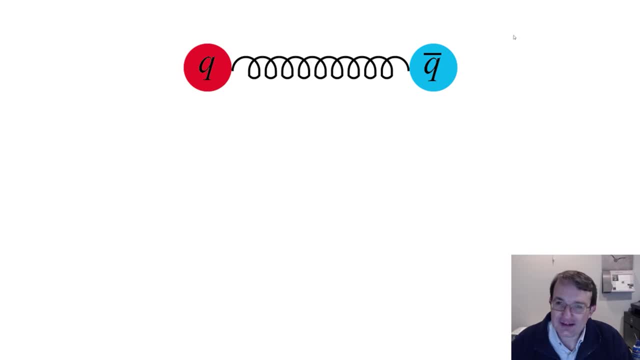 force. and what I'm going to do now is say: well, what happens if we add energy to the system? And so the way we can add energy to the system is, essentially, we're going to pull these two quarks apart. So, as we pull them apart, what's going to? 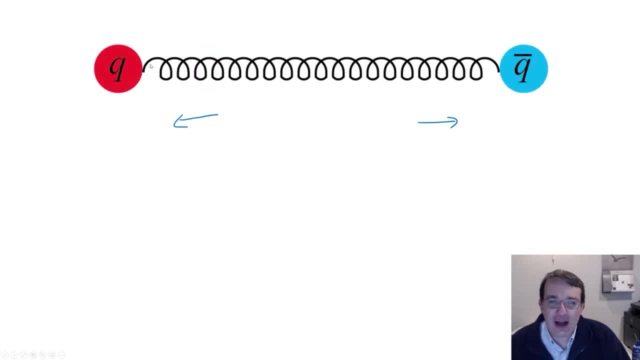 happen is this string is going to expand, And so now we get an expanded string and we've put some energy into expanding the string. Now the question is: what's going to happen as I keep pulling these quarks apart? What happens when the energy I have put into? 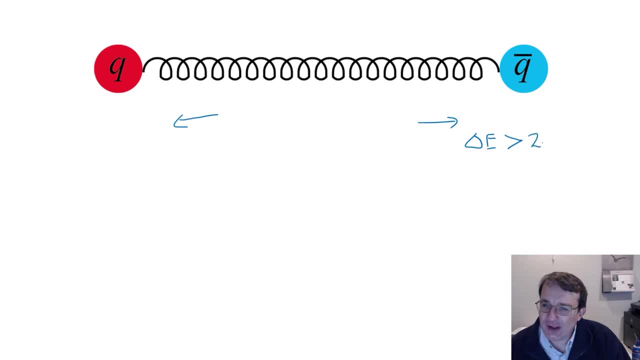 the string is greater than two times the mass energy of a pair of quarks. right, And these could be different flavors of quarks, but as I put more and more energy into this string, at some point I'm going to have exceeded twice the energy of the string. 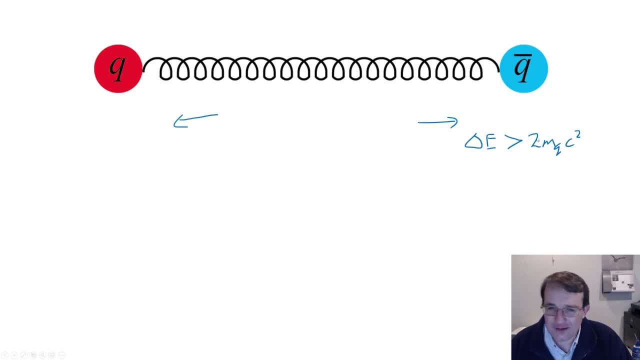 So I'm going to have an expanded string and I'm going to have an expanded string And that's the mass energy of a quark, of a flavor of quark, And when that happens, the string is going to snap And the energy in the string will get converted into a pair of quarks, because 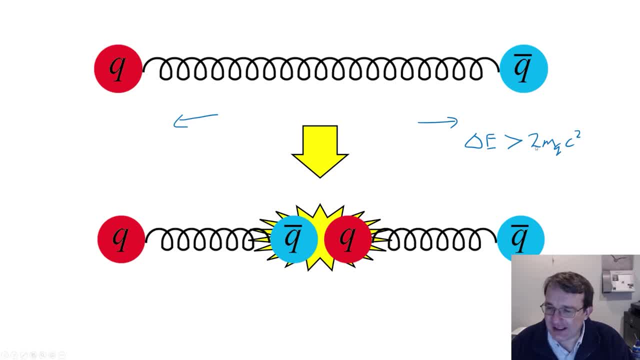 I've now, you know, I can convert the energy in the string into a pair of quarks And by because this will now allow the string to collapse right, So these quark-antiquark pairs can can move together. I have essentially it's energetically favorable for me to do this. 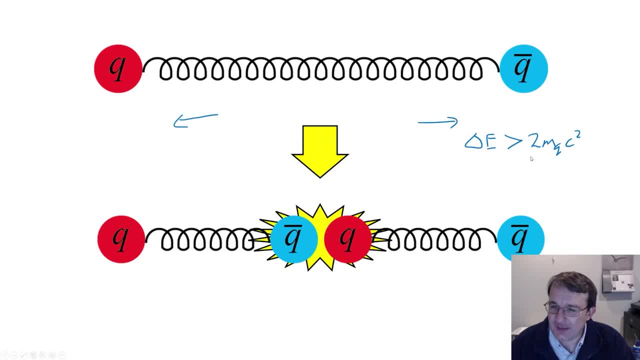 because the energy in the string is greater than twice the mass energy of the quark, And so once I've created a pair of these quarks, I've released more than twice. you know, I've taken away twice the mass energy, and whatever else I have left is now released. So it's. 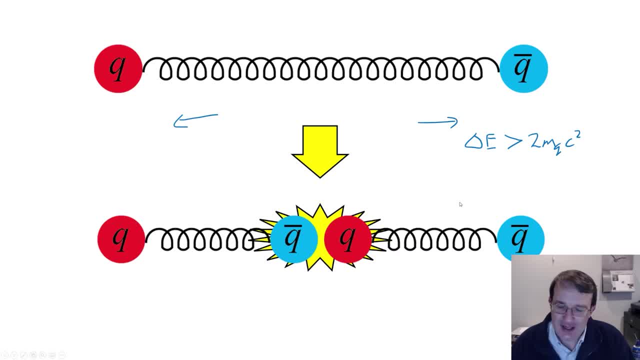 energetically favorable for this reaction to happen, And this is why you don't find free quarks. This is why it was impossible to knock out a free quark, because every time you do this instead, what happens is you just produce more mesons. So you start with a meson and you 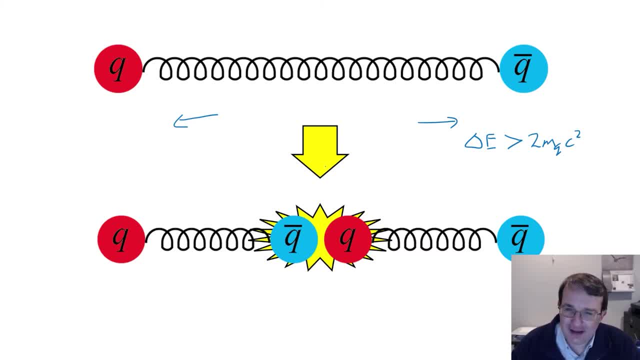 can do this with baryons too, And as you put more and more energy into it, at some point the string will snap and you'll produce quarks. And those quarks will rapidly bind up and you end up producing bound states of more mesons and more baryons. 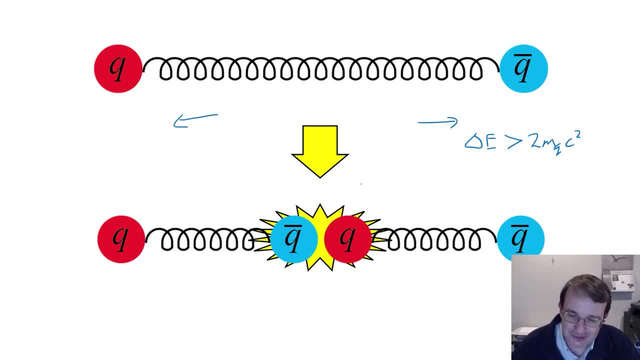 And you can actually. even starting with a meson, you can produce baryons too. I mean, obviously you have to produce a baryon-antibaryon together, but if you've got enough energy you can do that. 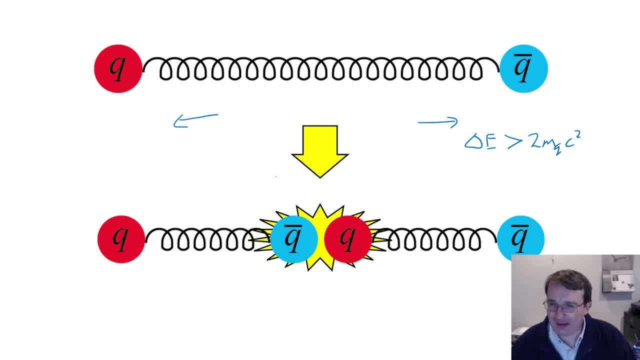 And so this is what happens: You can't separate the quarks, because the amount of energy involved separating them is way more than enough to just create more and more quarks, And so all you end up doing is just creating more and more hadronic particles. 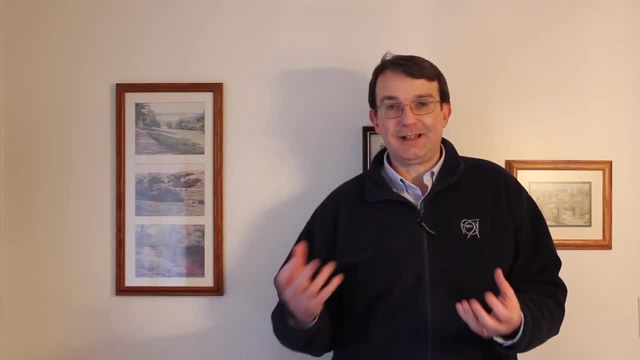 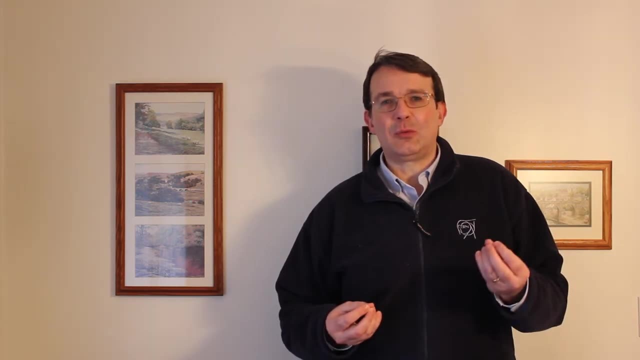 Now, confinement means that when we produce a quark, or indeed a gluon, we're going to produce a baryon, And that means that when we produce a quark, we're going to produce a baryon in a high-energy collider. We don't see that quark or gluon. Instead, what we see. 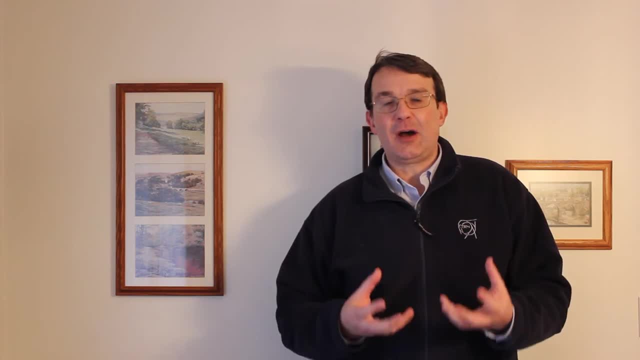 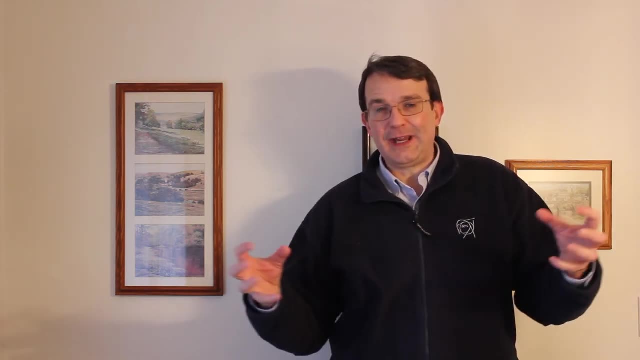 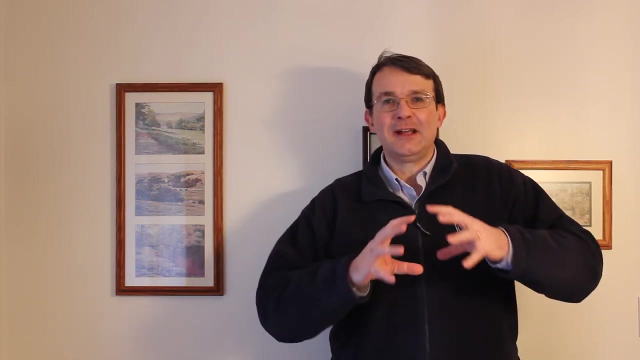 is a jet of hadronic particles that come from that original quark. What happens is just as we've shown: the string or spring stretches until it snaps and produces lots of quark-antiquark pairs, which all bind together to form different types of hadrons, Mesons, baryons, mesons. 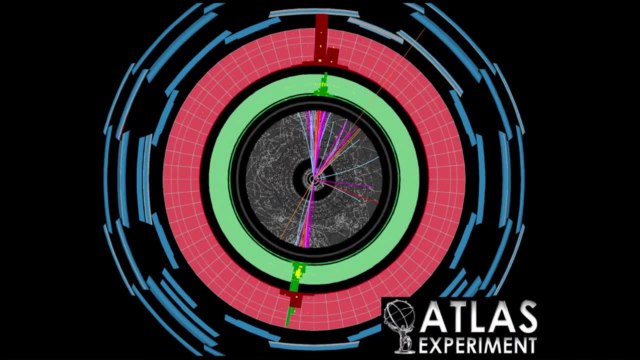 and anti-baryons. However, because momentum has to be conserved, the particles that all come from the original quark will all be boosted along the momentum direction of that original quark, And so you get these collimated jets of particles such as this one that we can. 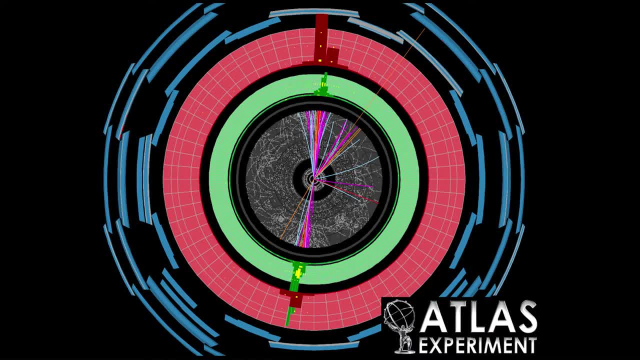 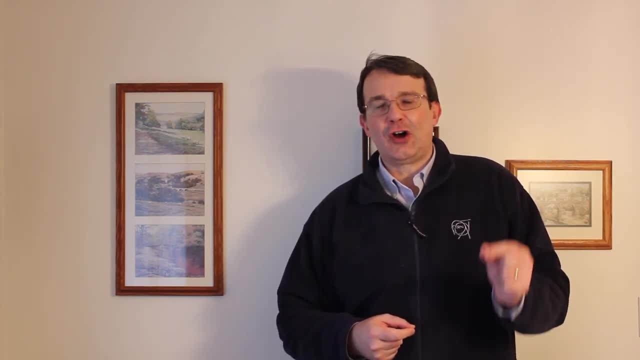 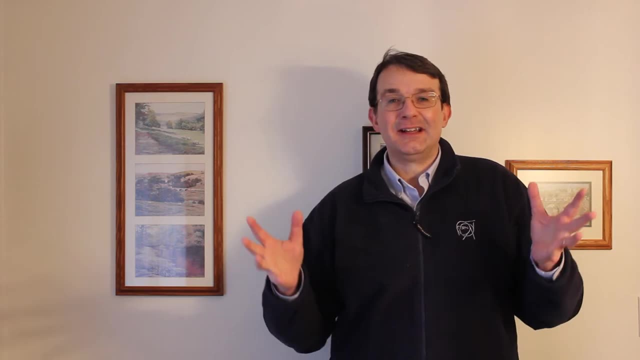 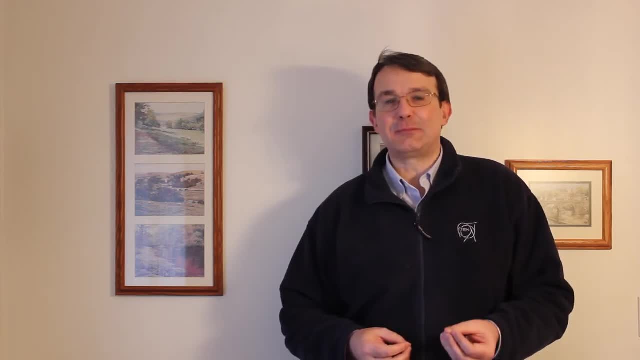 And so that's actually one way that we can study the properties of a quark that's outside a bound state, simply because it doesn't live long enough to form a bound state. Now there is another way that we can remove quark confinement, but to do that we have to turn up the temperature a little bit. 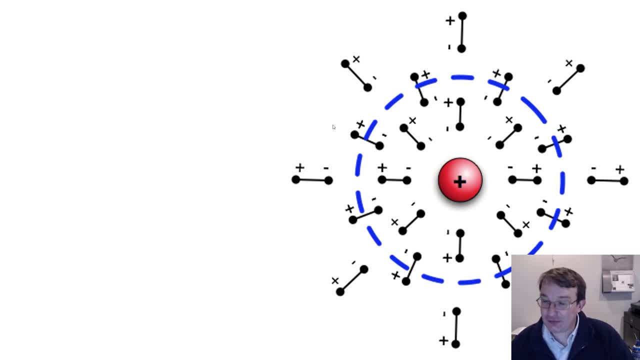 Now to understand what happens in renormalization and how things change with energy. let's have a look at a simple classical example to start with. So what we've got here is we've got a positive charge and we put that positive charge in water. 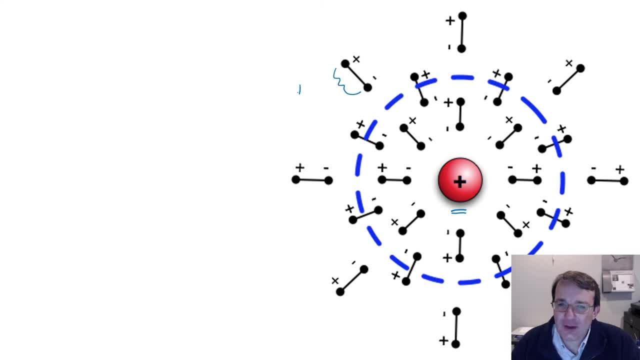 And water consists of a dipole molecule. so this is our H2O molecule and it has a positive end and a negative end, And what happens is, if you've got a positive charge, the negative ends of the molecules will point towards. 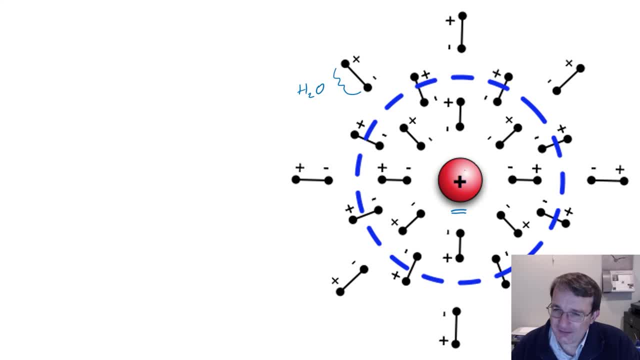 or tend to point downwards. It's more likely to point towards the positive charge, and the positive end, of course, is going to point away because it's repelled, And so you end up with these dipoles all around the electric charge. 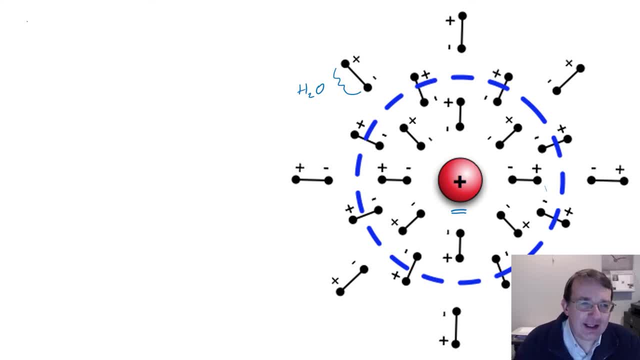 Now, if I have this electric charge in vacuum, then we could look at the electric field due to this and this would be equal to the charge over 4 pi epsilon naught times R squared, And that would be the. That would be the electric field strength for an electric charge. 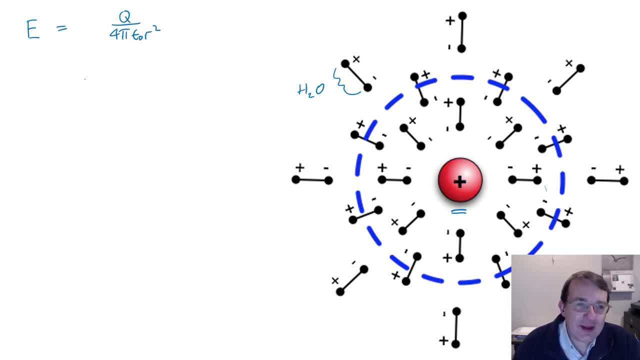 Now, if I put that charge into water, then my electric field changes and it becomes Q over 4, pi, epsilon, R. epsilon naught, R, squared. So epsilon naught here, of course, is the relative permittivity of free space. 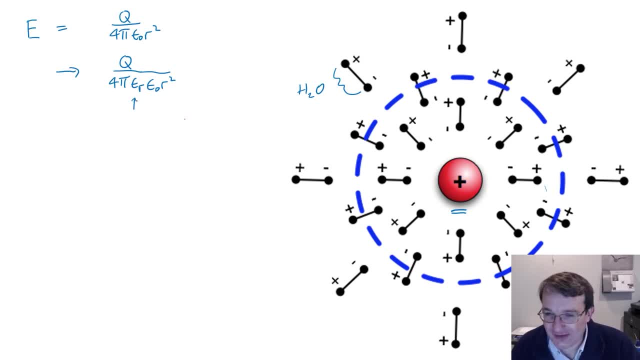 and this is the relative permittivity, And this is the relative permittivity of water right compared to that of free space. And so what this means is is that the electric field is going to be less because all of these water molecules here are shielding the positive electric charge. 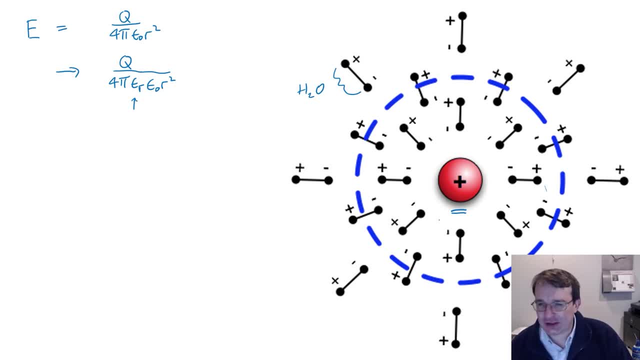 The electric, The water molecules shield the electric charge. Now, what happens in a vacuum is exactly the same. Instead of these things, Instead of these things being water molecules- they are, in fact, positron-electron pairs that pop out of the ether. 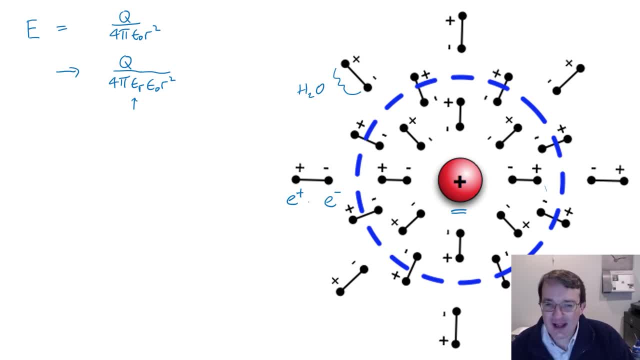 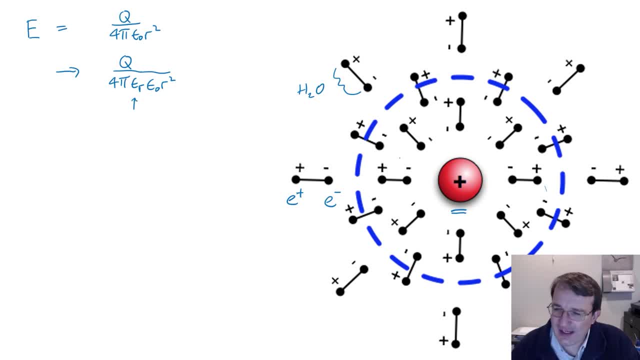 The positron is going to be, you know, preferentially further away, But the effect is the same: A vacuum will shield an electric charge. So what does that mean? Well, if we're measuring the electric charge or the strength of the electromagnetic interaction, 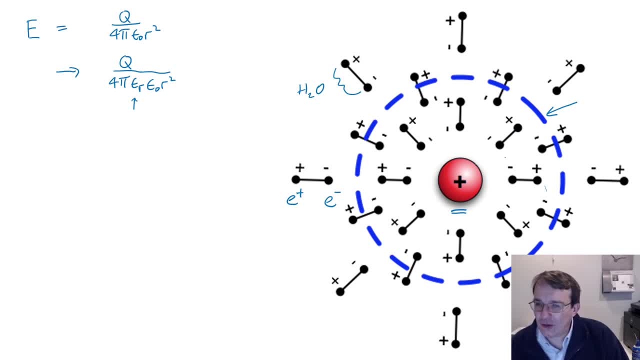 at the distance of this blue line here. then we have all of these guys who are shielding the charge because they sit in between us and the positive charge. But if we now move that ring in, then instead of measuring it at this distance, 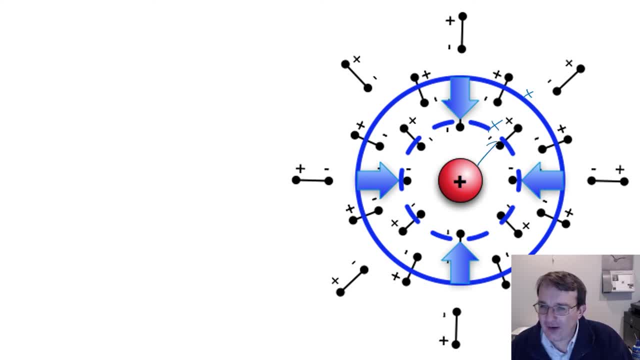 and we measure it at this distance, then now we have far less, far fewer electron-positron pairs that are acting as insulation right. So we have, as we go to smaller distance scales. then we have less vacuum in the way. 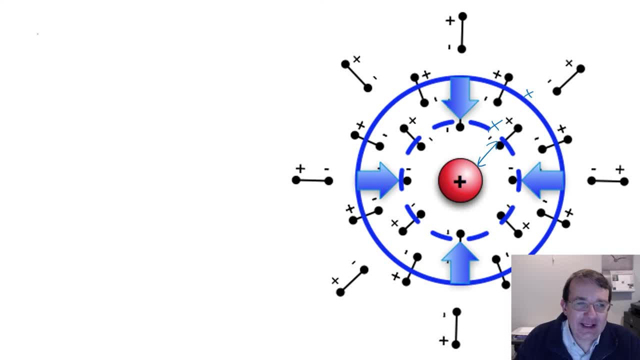 shielding the electric charge, And so what that means is that the strength of the electromagnetic interaction increases as the distance scale decreases. Now another way of saying: the distance scale decreases. if you want to probe very, very small distances, you have to go to higher energies. 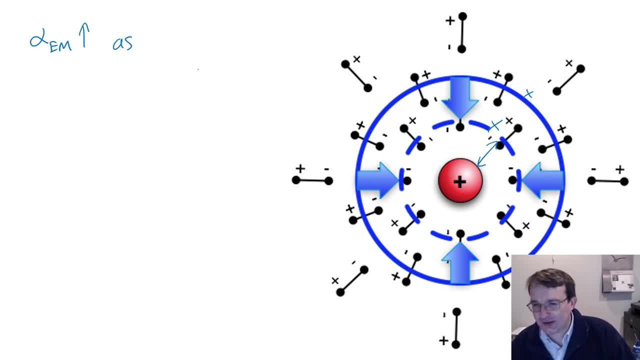 because you need shorter wavelengths of particles to probe those very, very short distances, And so a shorter distance is exactly the same as saying a higher energy, And so what you find is that there is a correlation between the strength of the electromagnetic force and the energy at which you're probing things. 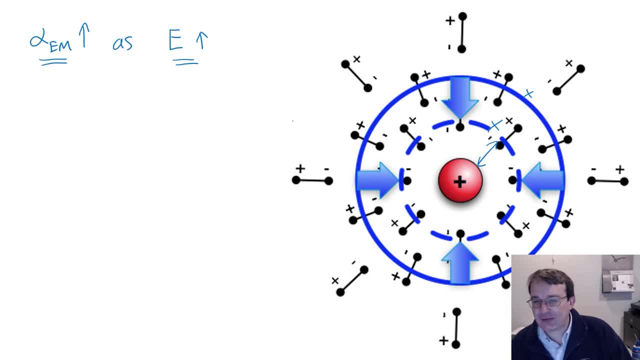 And as you go to higher and higher energies, the electromagnetic force gets stronger And in fact we've observed this. the fine structure constant measured at the Z, the Z boson mass, is very noticeably higher than it is when you measure it in sort of classical experiments. 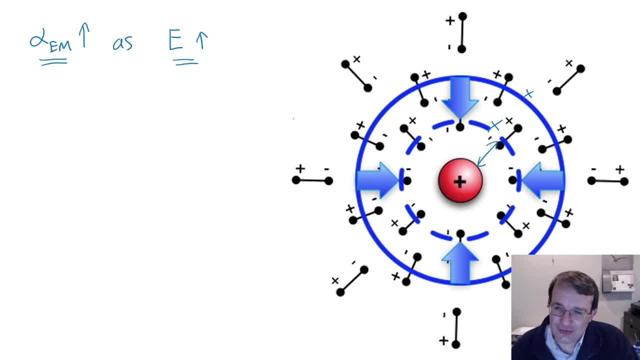 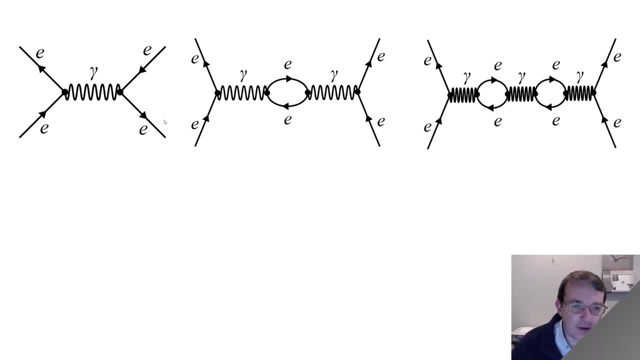 at very low energies in the lab. So this is a proven effect. So how do we represent that in a Feynman diagram? So here are the Feynman diagrams that represent that process we just talked about for electromagnetism. Here's our tree level diagram. 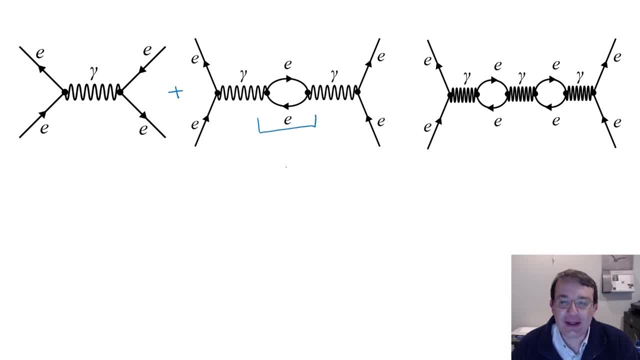 And then we add to that. we can put- we can put a loop in here- And in fact we saw that, you know, when we were looking at higher order diagrams- Then we can add to it, we can put two loops in here. 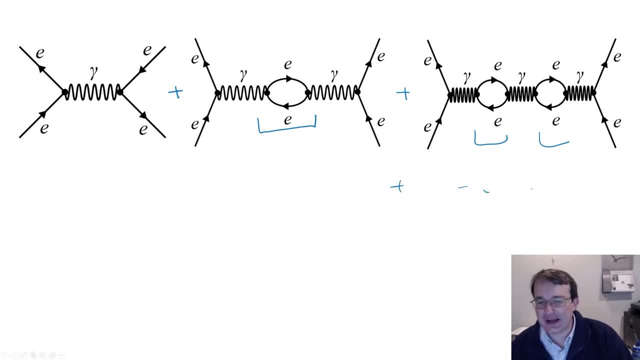 And of course you can carry this on with three and four and five and any number of loops, And so that is how we can represent renormalization in Feynman diagram form. So how does this look for the strong force? So here are the Feynman diagrams. 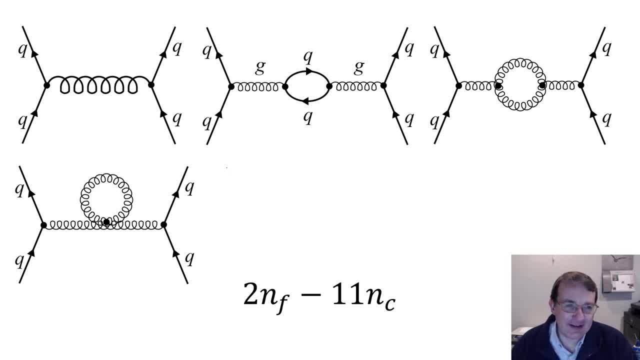 for the same process in QCD, And you can see that there's quite a difference. So here is our tree level diagram, where now, of course, we have to have quarks And instead of a photon we have our gluon. Now the one that looks like the diagram from QCD is this one. 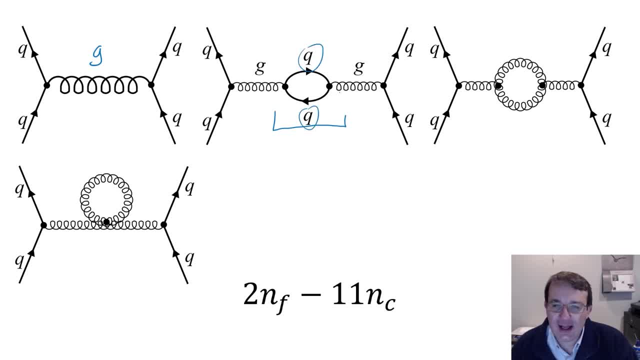 where we have our nice sort of quark anti-quark loop between two gluons, And so that looks very similar. But because the gluons can couple to other gluons, we have two other possibilities. So here is our three gluon vertex on either side. 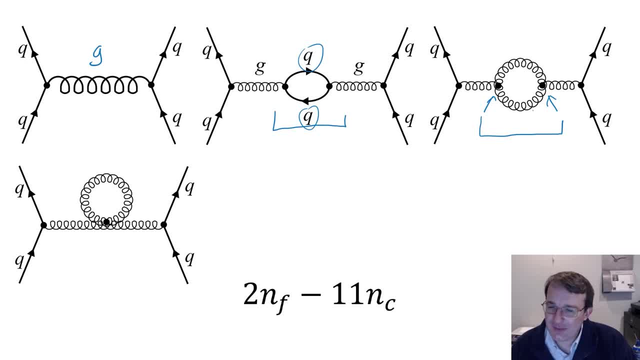 And so we can have this sort of gluon loop in the middle of the propagator, And here we have our four gluon vertex, giving us this rather sort of funny thing where we have a loop that looks like it's completely disjoint. 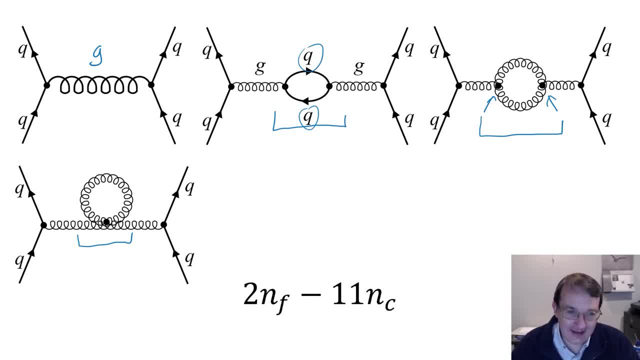 but this is a valid diagram and you can calculate it and it has a contribution to the process, And so you've got far many more ways in which you can contribute to how the strength of the force changes, because gluons couple to other gluons. 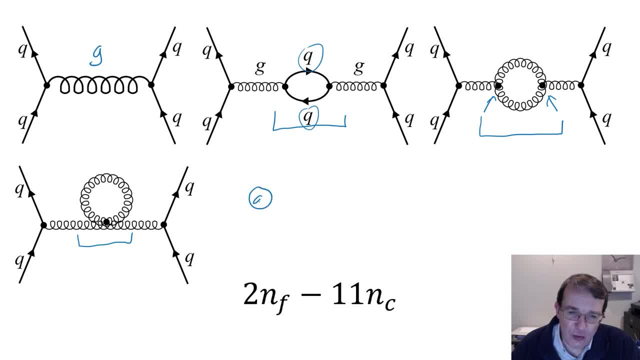 And so, if you sort of think of this, in our picture of a quark sitting in the vacuum, it's not just surrounded by quark anti-quark pairs, it's also surrounded by funny gluon loops that are bound together in different ways. 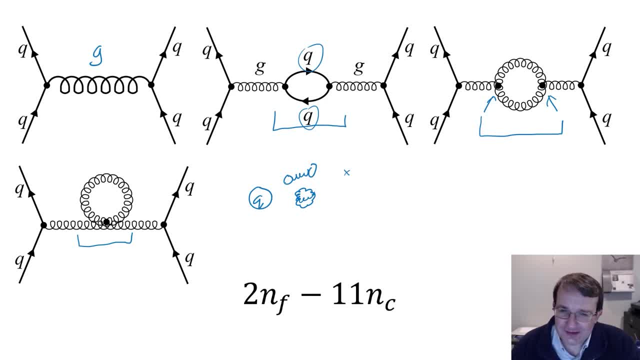 And so when we're sitting out here, we don't just see quark anti-quark pairs, we see gluons as well, And in fact, even in the quark anti-quark pair we see the gluon, because the gluon has a color charge. 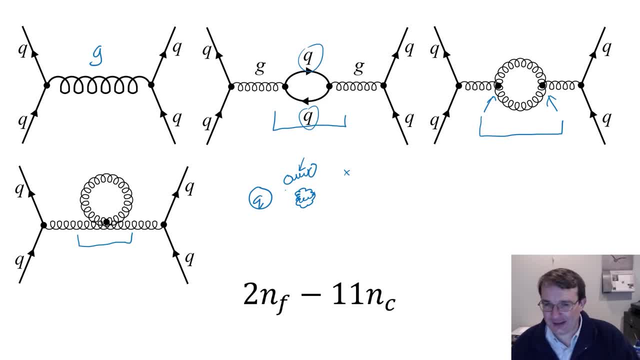 Now for these models, these sort of QCD-like models, where you have the carriers, where the force carriers themselves carry color charge. you end up with the overall change in the force, depending on an expression that looks like this, Where Nf is the number of quark flavors. 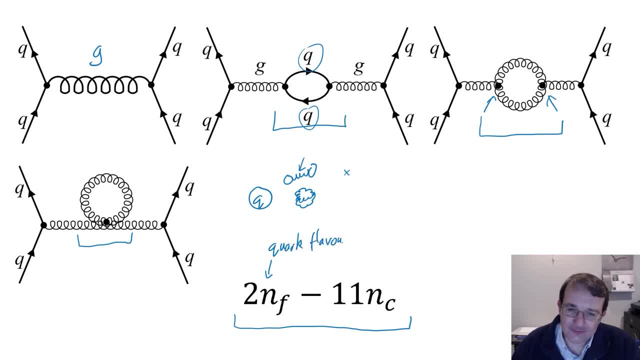 So this is quark flavor here And Nc. here is the number of colors, And so if you put the numbers in for QCD, well we have six quark flavors. So this is equal to six And the number of colors is equal to three. 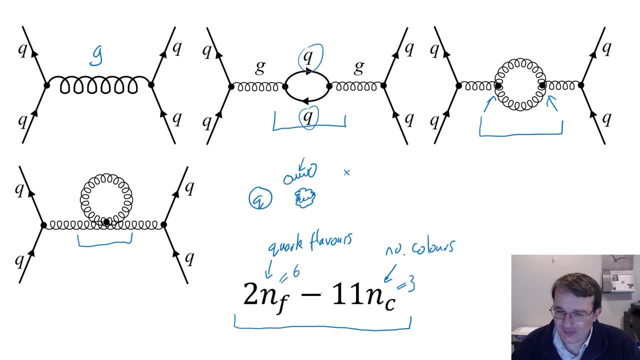 And so you can see that you end up with something that's negative. Okay, And so what that means is that QCD behaves exactly opposite to electromagnetism, And so the strength of the strong force decreases as the energy increases, And the way you can think of this is that all of these color 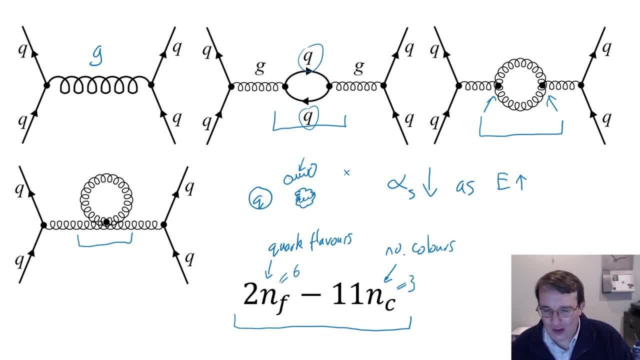 you know, the fact that we've got this- you know quarks and gluons and we don't- we're no longer just sort of seeing the virtual quarks, we see all the virtual gluons as well- means that all of these sort of different virtual things- 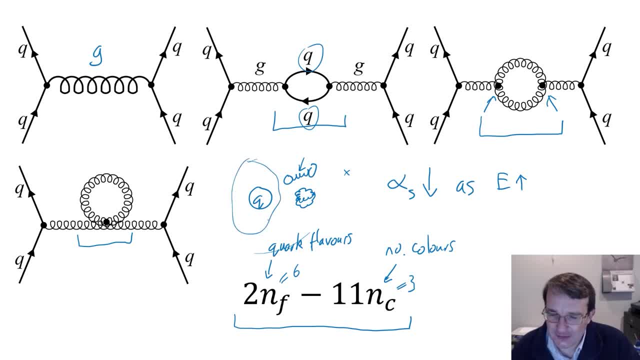 that appear around our quark in the vacuum increases the strength of the quark's charge, And so as you go to higher energy and you get to shorter distances, you see less vacuum. There's less vacuum in there, So you see fewer of these virtual things. 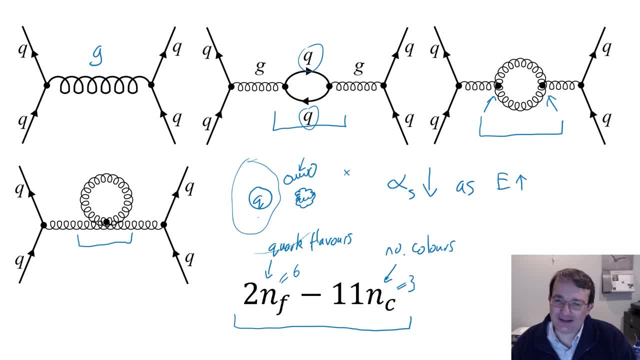 popping out of the ether, And so the charge on the quark appears to get less, or rather, the strength of the strong interaction gets less and less and less, And so we have something that's called asymptotic freedom, that, at very high energies, 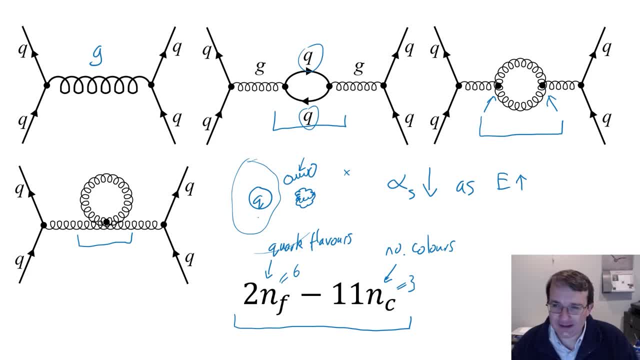 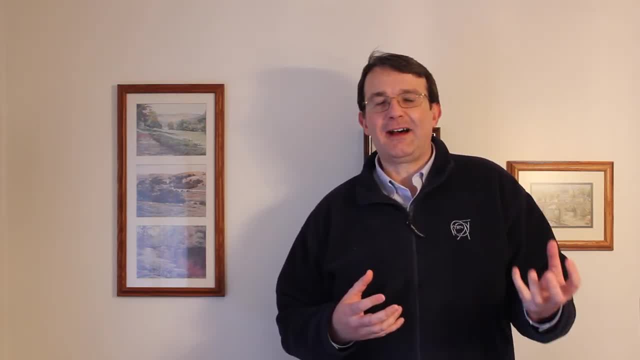 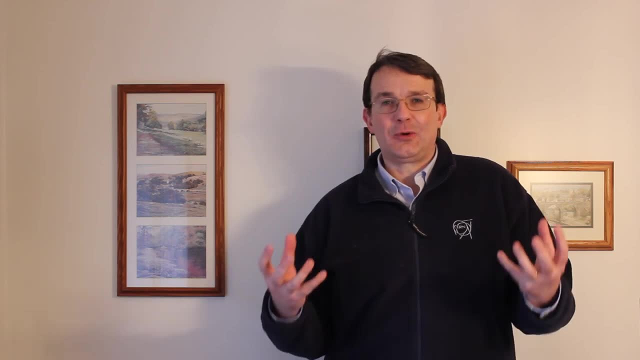 the strong force actually becomes very weak. So what this renormalization means for the strong force is: as we go to higher and higher energies, the strong force becomes weaker and weaker and weaker, And we get what's called asymptotic freedom. 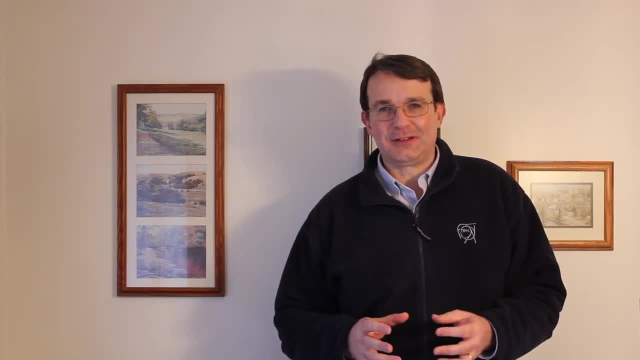 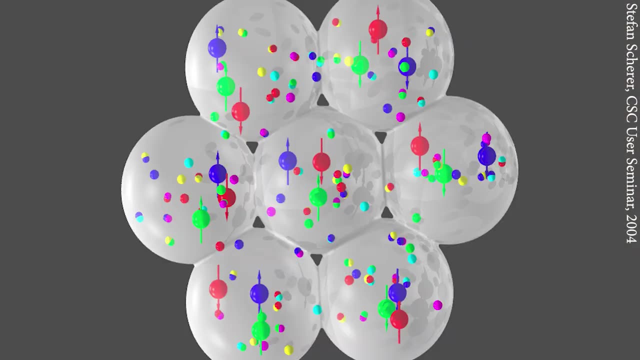 In the limit of infinite energy, there's no strong force at all. In practical terms, what this means is that if you turn up the temperature high enough, you heat up matter sufficiently. then the quarks in their bound states, these bound states, the baryons and the mesons, 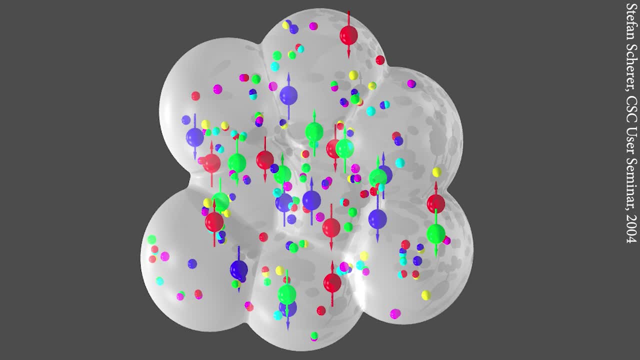 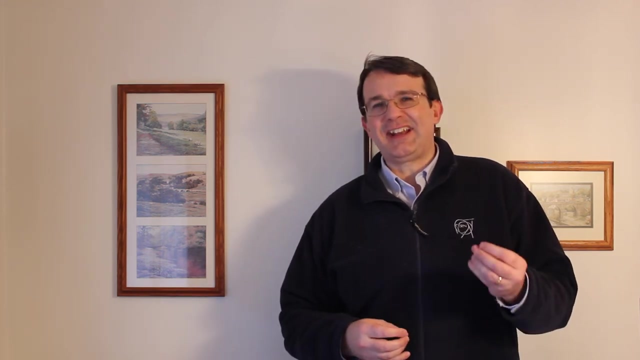 will literally melt, And they will melt to form what's called a quark-gluon plasma, And this is something that has been theorized for quite a while, and we do now have experimental evidence for, However, that experimental evidence was extremely hard to get. For decades now people have been studying the collisions, particularly for sort of heavy iron collisions, where instead of colliding a proton on a proton with an antiproton, you're colliding essentially one heavy iron with another heavy iron, and so you have many hundreds of nucleons. 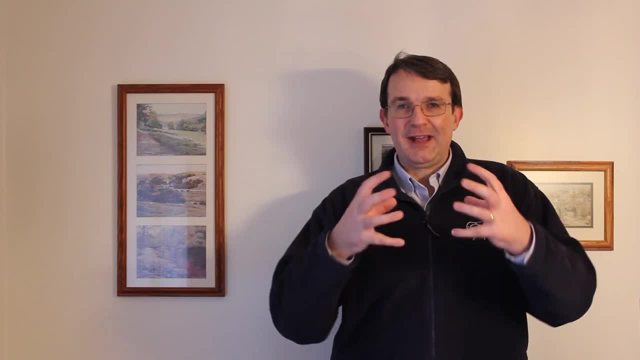 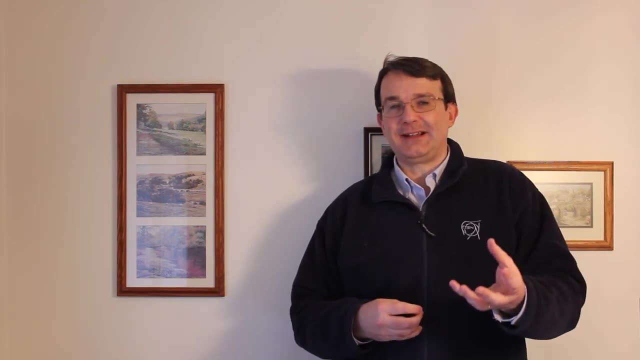 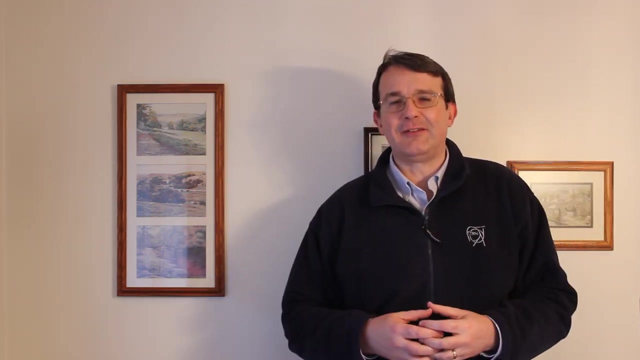 involved in the collision so that you have a significant volume of superheated matter. And when people have been doing things like that or doing collisions with heavy ions, collisions using fixed target heavy ions, there's been a whole series of trying to. 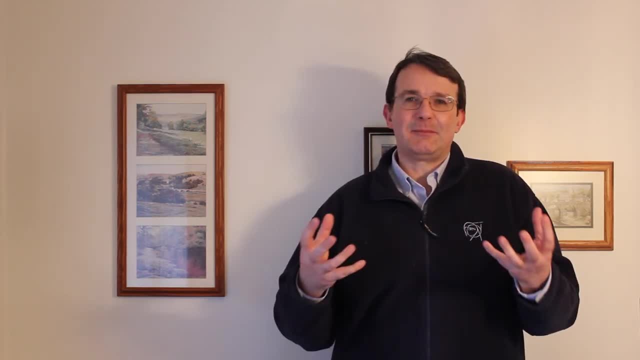 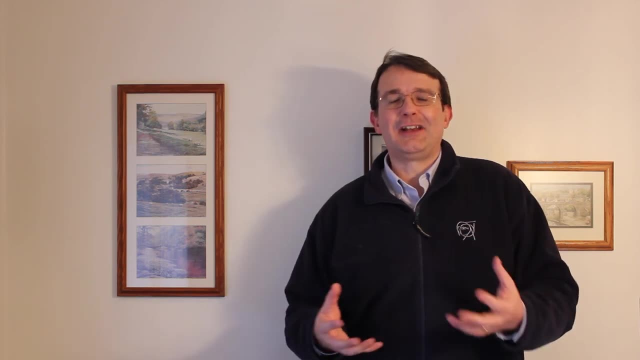 come up with theoretical predictions, measurements they can make to prove that a quark-gluon plasma has been produced- And this has been, I would argue, at least has been- a contentious issue in the field with, for quite a while, people not being 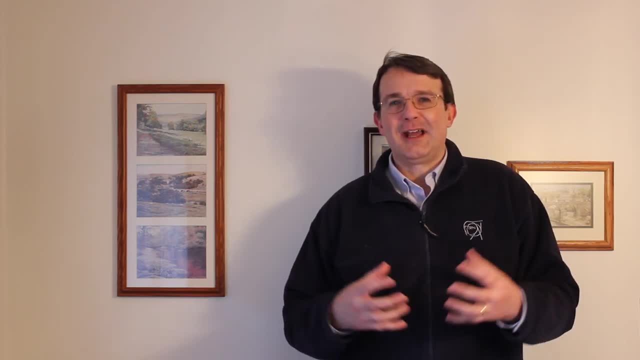 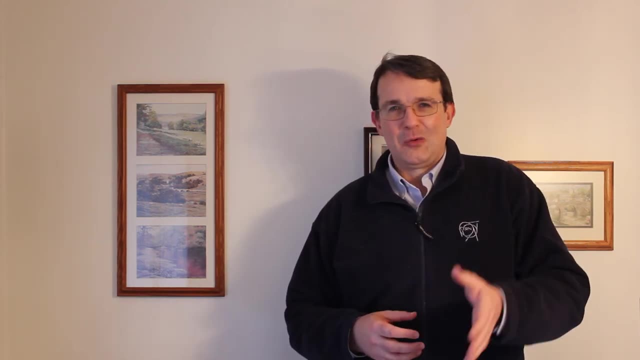 really quite convinced that quark-gluon plasmas have been produced. I think the Wikipedia article says they were first produced in 2000.. I've certainly been at conferences well after the year 2000, where people were still, you know, asking the question of. 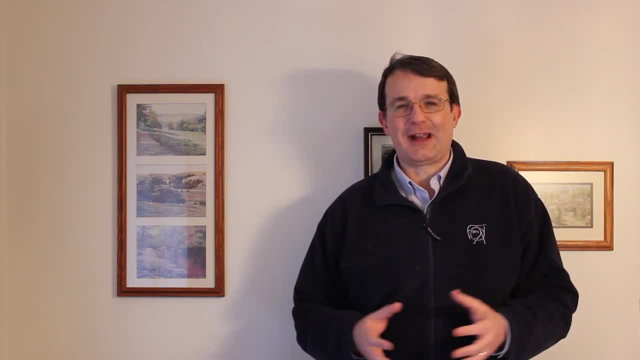 well, is there ever going to be any conclusive evidence that quark-gluon plasmas have been produced? Well, now we do have conclusive evidence that quark-gluon plasmas have been produced, and that evidence actually came from. 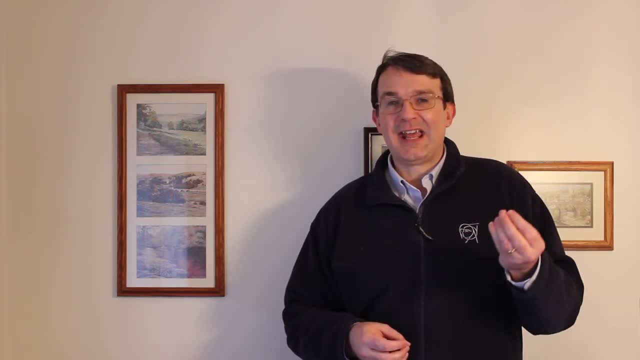 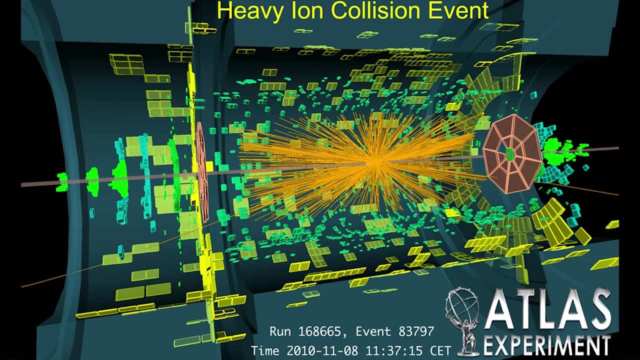 the Large Hadron Collider with its first heavy iron collision run. So this was in November 2010,. when it was running with lead ions, colliding with lead ions, And when this happens, of course, you get all these hundreds of nucleons. 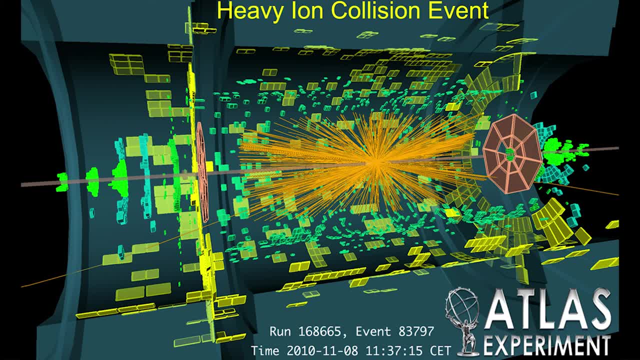 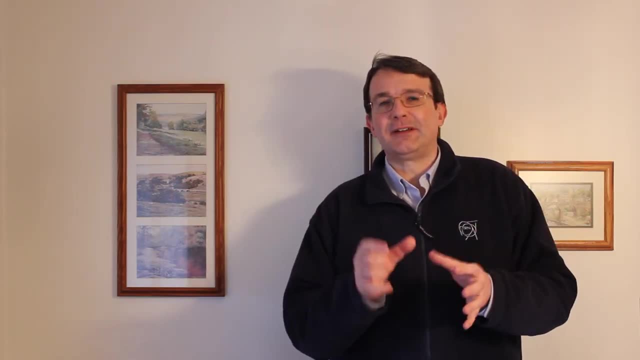 colliding at incredibly high energies- Not as high as two protons in the Large Hadron Collider, but nevertheless well- at multi-GEV energies per nucleon, Multi-TEV- sorry- energies per nucleon. And when this happens, if you have, 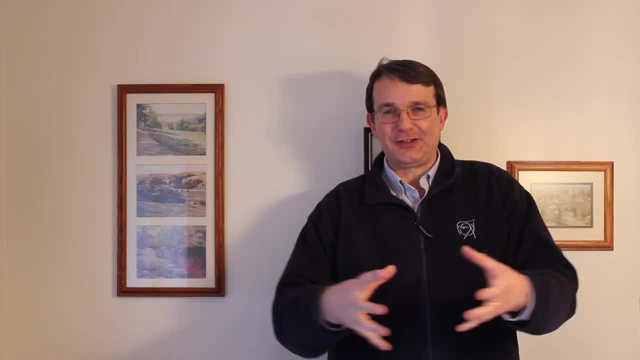 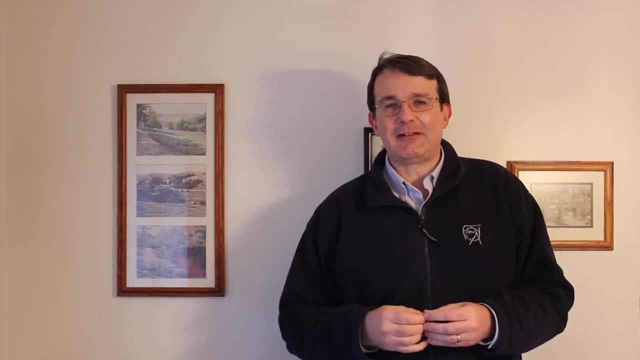 a pair of nucleons on the edge of this sort of huge fireball, then if those two nucleons have a high energy interaction, then just like any pair of high energy, just like any pair of protons colliding that have a high energy interaction, 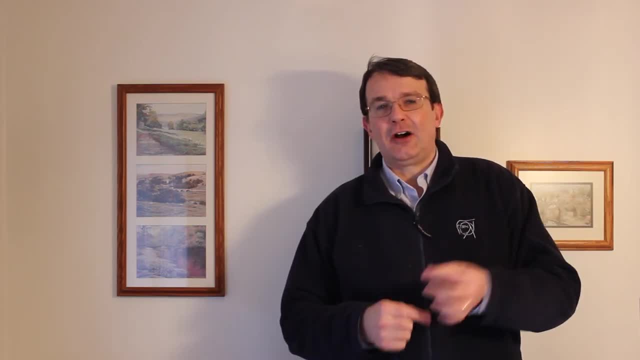 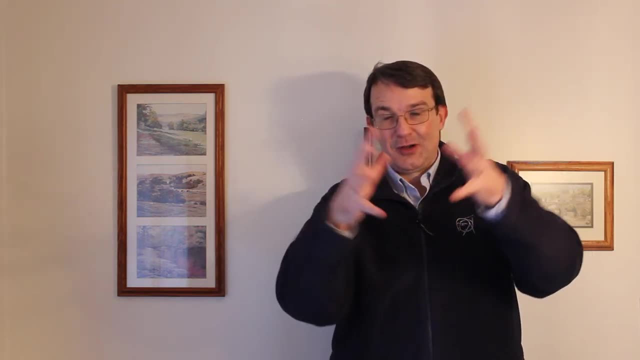 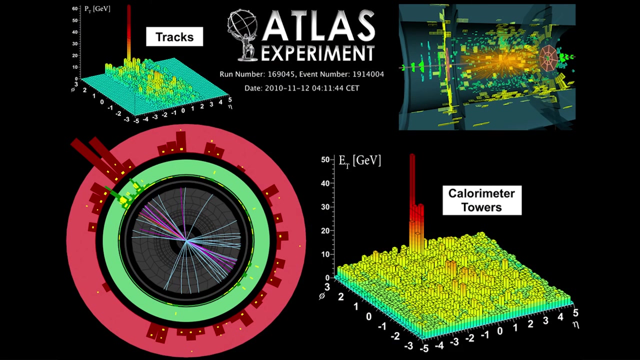 they will produce two back-to-back jets of hydraulic particles. But these two jets are back-to-back on the edge of this. you know nuclear fireball in the middle of the detector And what happens is one of the jets will shoot out of the edge of this fireball. 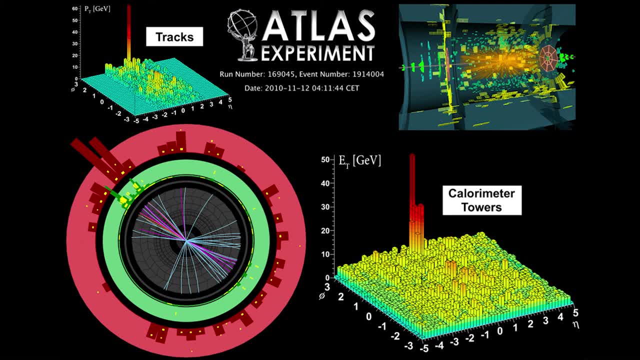 and you see that, as a high energy jet, The other high energy jet goes into the fireball and because it's this super dense quark-gluon plasma, that plasma essentially absorbs the energy and momentum of the jet. So what you see is on one side of the detector. 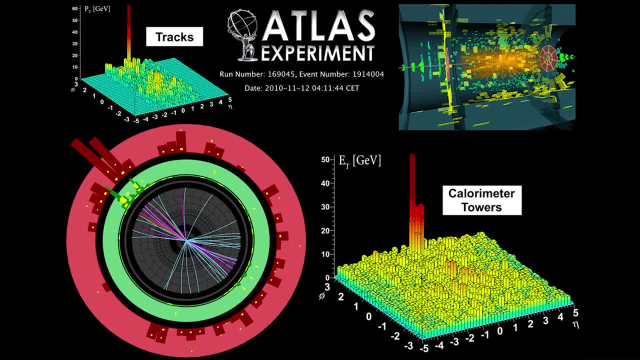 you get this high energy jet of particles and on the other side of the detector you get a balancing amount of energy and momentum. but instead of being in a very collimated beam of particles, it's spread out over half of the detector, And that's because the energy 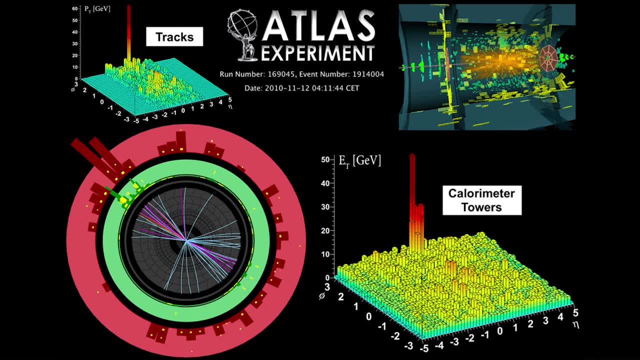 has been lost from the jet and transferred to this quark-gluon plasma, And the only way to explain these events is by the formation of quark-gluon plasmas, And so everybody is now convinced that we have produced quark-gluon plasmas. 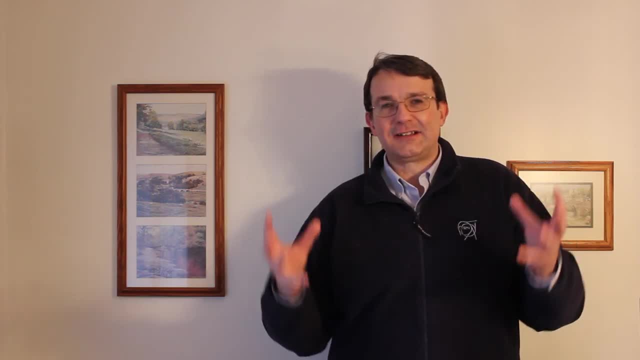 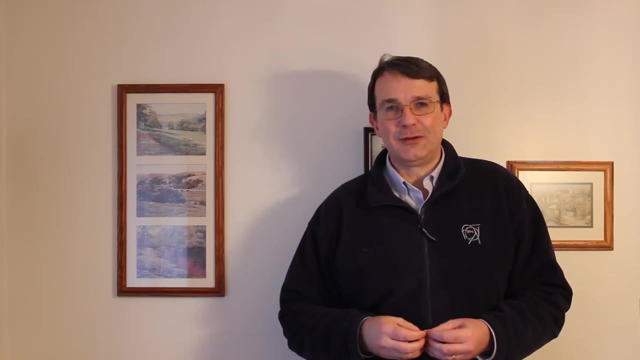 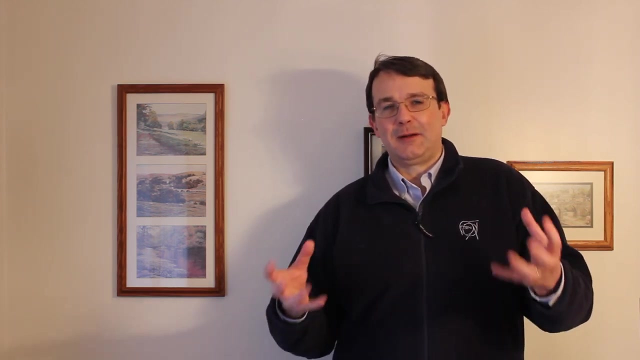 and in fact there's a whole research industry studying the properties of this, because it turns out it's very, very close to an ideal Fermi fluid and so it has many interesting properties. It's also critical to understanding the very early universe, because up to about, 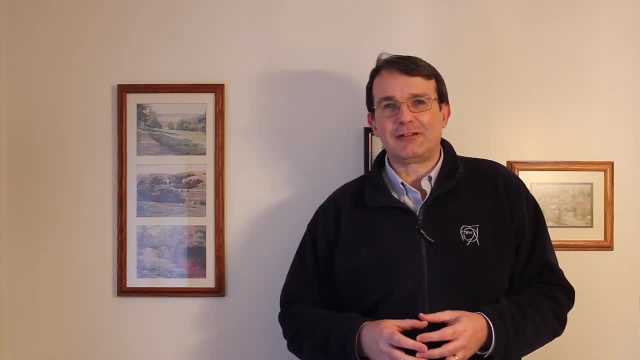 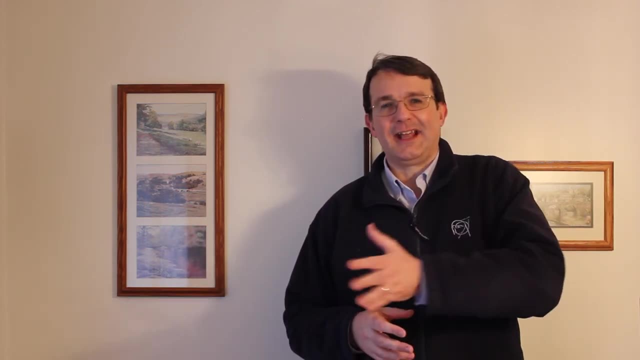 10 to the minus 5 seconds, so just over a microsecond. that was where the big bang was. it was quark-gluon plasma. After about 10 microseconds then it cooled down below that temperature and we had the hadrons form.